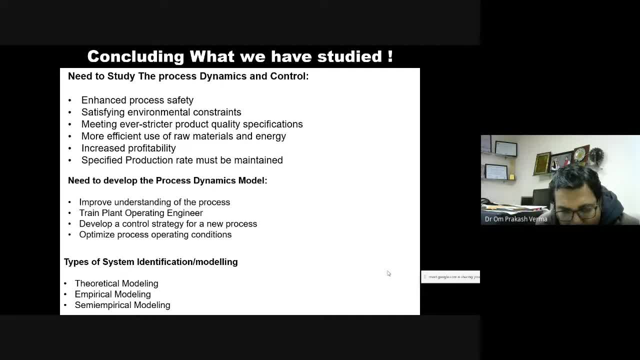 Okay, Second is the empirical modeling. Empirical modeling is based on the dynamics, So it is based on the data science, data analysis, whatever the history of the data is available, in the of the, any equipments, or in the plant or of the industries, based on that data, of that particular equipment or the industries, or the something else. 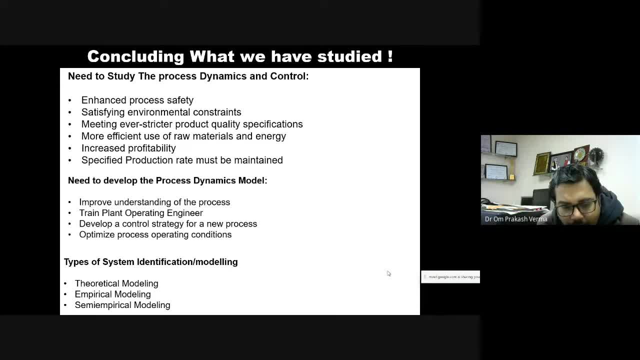 We are trying to find out the behavior, future behavior or anticipate the behavior of the system based on that data. So we have to develop the model using that empirical model. Okay, That data. So it will require a statistical tool. 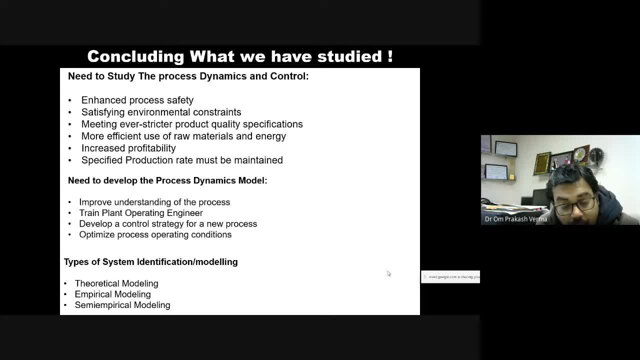 You have already heard about the- you know- RMX model, autoregression model. We will study this model in the DSP Distance Signal Processing. Next, the semi-empirical modeling. Semi-empirical modeling comprises of two words. 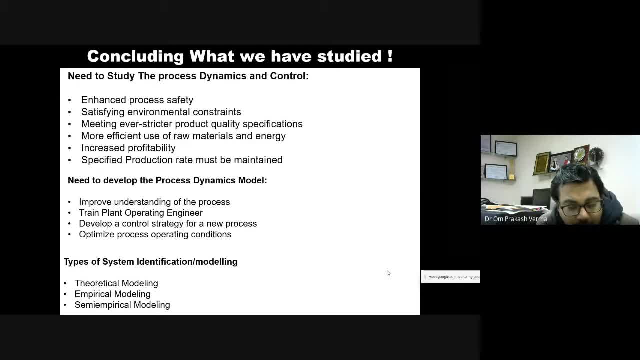 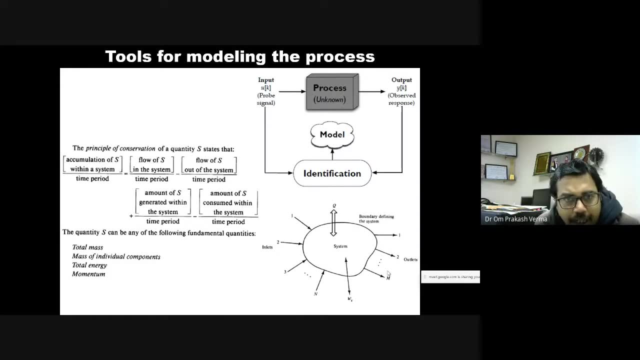 First is semi, and then semi And empirical. it means it also uses the theoretical modeling as well as the empirical modeling. We will see, with some example, how these three models will going to develop. So first model, first tool is the theoretical model. 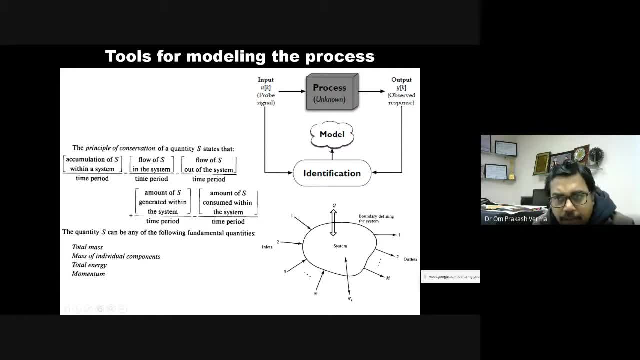 And in order to find out the theoretical model- you can understood it, how it is will be When we going to apply some input, input signal to the any process. Obviously it will generate some output And this output we have to find out how this output is going to behave. 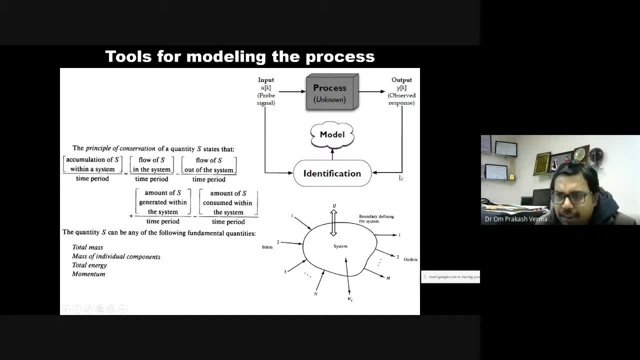 Okay, So we have to measure this output And the output. we have to find out the relation between the output and input, How this output behaves with the basis of this input. Okay, So we have to model These things using some mathematical tools. 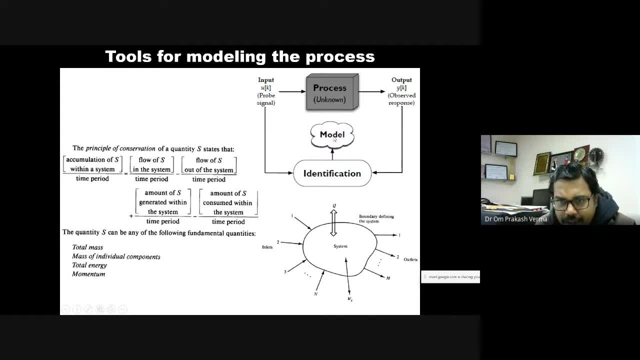 So this term is known as identification, or the mathematics dynamics we got is called the model. Okay, So these are things. So what are the different things? What are the different tools? So first theoretical tool is the principle of conservation. 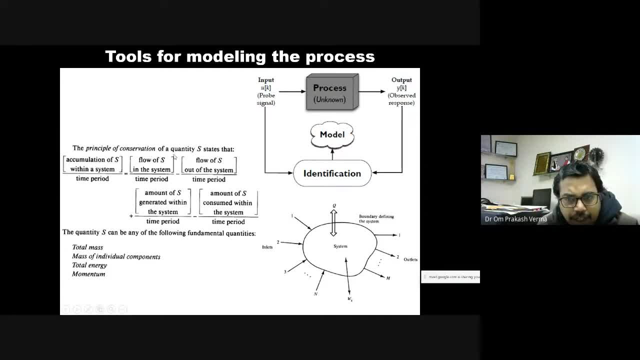 So principle of conservation means principle of conservation means whatever you send the items inside the system is equal to the whatever the items leaving the system, Is it okay? So based on this, you can say that the accumulation of S within a system 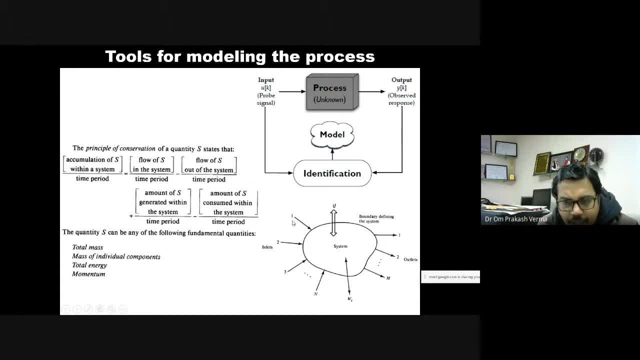 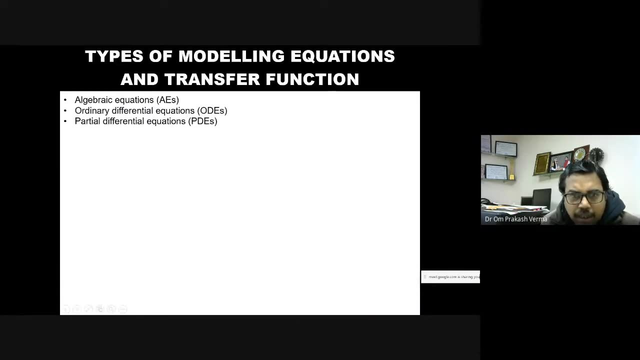 Accumulation of S within a system means whatever you are sending is equal to the accumulation part. Whatever you let's say, suppose there is a tank And in a tank I am. I am giving one example so that you can understand it. 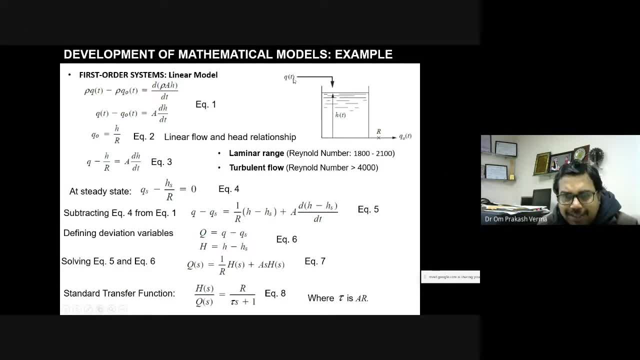 Let's say there is a one tank. In this tank let's say you are sending some some, some fluid or some water inside the tank And this is the. this is the leaving part where the items are Okay output of there. we are getting the product okay. so let's say we are, we are sending some water. 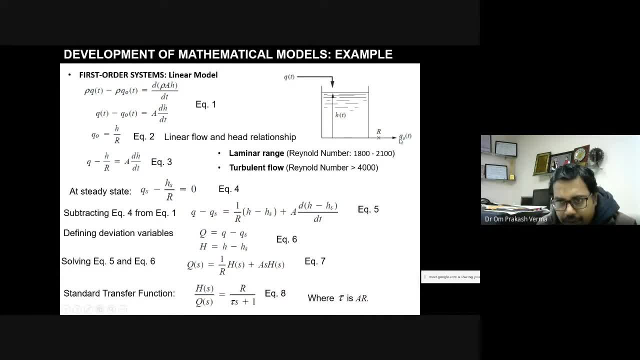 inside this tank and leaving this. living the this tank, uh, living with the help of this tank. so, whatever the, some water is going to accumulate here. that is the accumulation. so let's say we are sending 10 kg of water, so and 2 kg of water is living from this side, so 2 kg plus, whatever the. 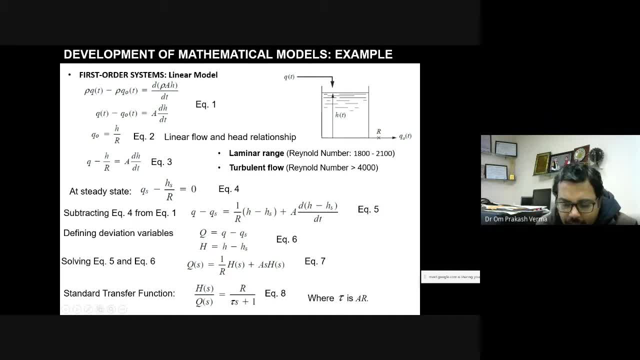 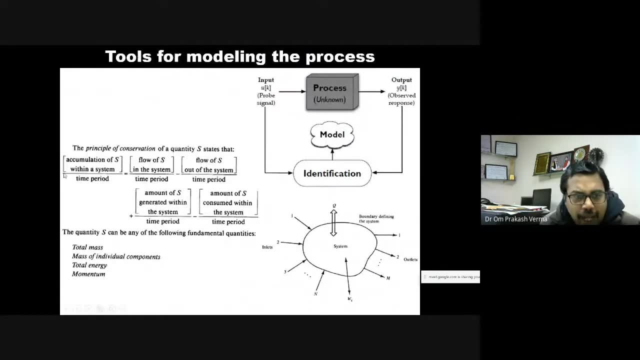 8 kg is going to accumulate. it is equal to 10. is it right? so you have to do this, you have to understand. so this is the, this is the accumulation. accumulation is equal to the. whatever you going to set the in minus out, or you can say in equal to the out plus accumulation, both are the. 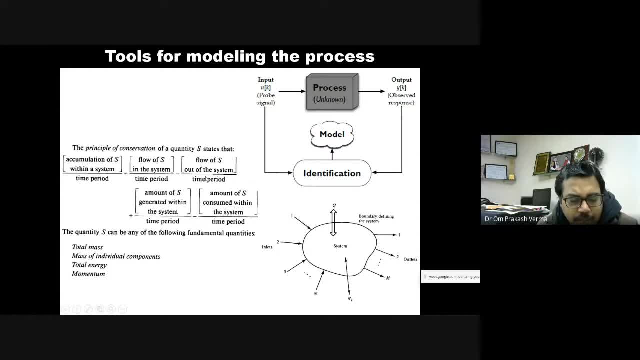 same. in is equal to the out plus accumulation. any doubt, any doubt up to this point. in is equal to the accumulation plus whatever, the out, okay, plus the amount of s generated within the system. let's say the system is. now you can say, uh, uh, what do you say? it has two words in the chemical. 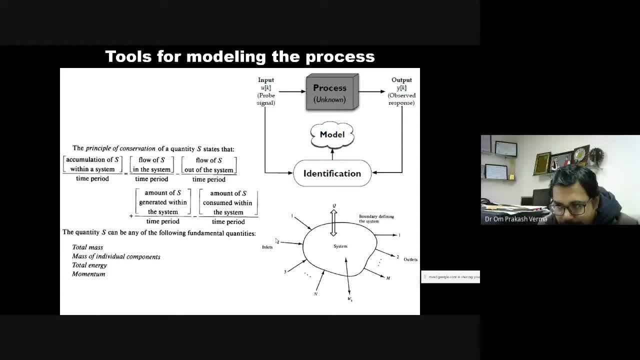 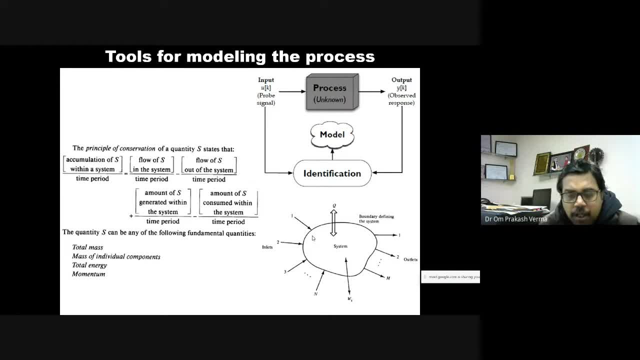 exothermic. that is the heat, basically the heat transfer. whatever suppose that you are, you are mixing two chemicals, a and b, okay, and some amount of s or some amount of salt, some amount of third part. third thing is going to generate it with this in the, in the system. 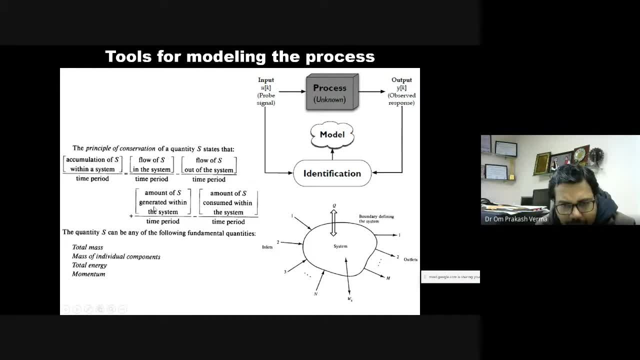 okay, so that is going to also add it right and whatever let's say, you are, you are, you are supposed, you are going to mix two chemicals and one came and some amount of chemicals are going to consume within the system. that, with the minus, whatever the generated is, a plus, whatever the system. 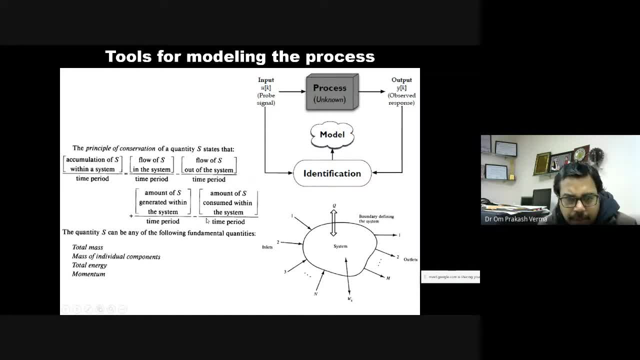 whatever is consumed, there's a minus. simple principle is: whatever the system is going to, the in equal to the out. in is equal to the out. that's the principle, that's the conservation of the system, something, anything else. it may be the mass, it may be the components, it may be the total energy. 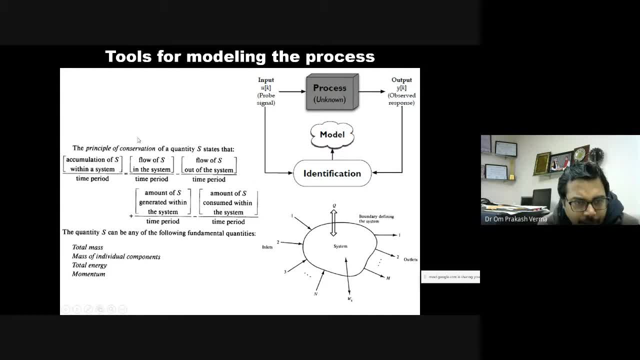 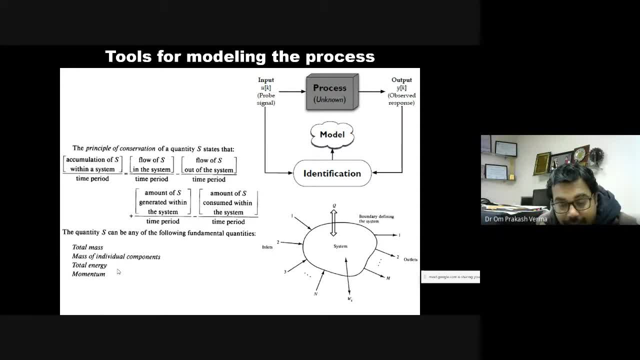 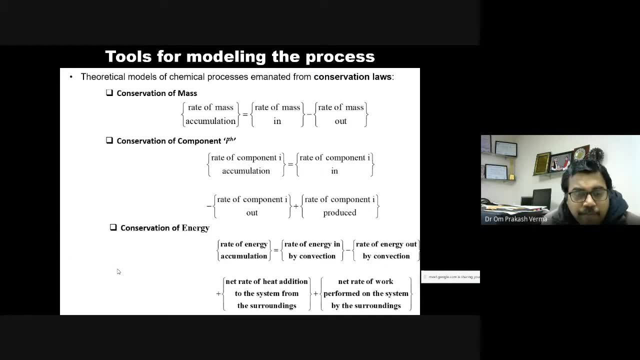 end of the reaction is exothermic, then heat is that. heat is, you know, generated and you have to add this energy. right, we will see with example how this will be detailed. so this is the theoretical model for the chemical process emanated from the conservation law. first you are seeing the 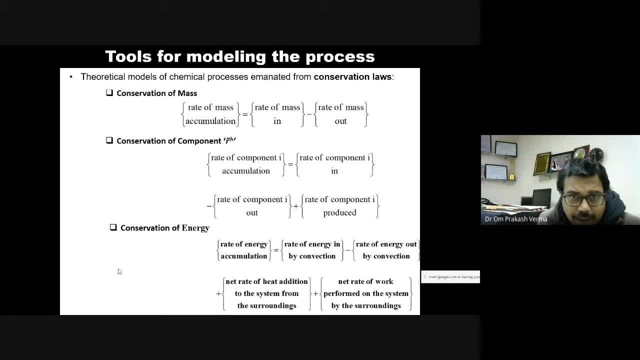 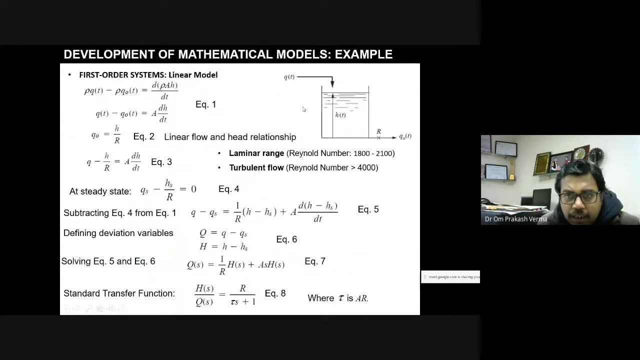 conservation of mass. in order to find out the conservation of mass, you can see here rate of mass, whatever the accumulator is equal to, accumulation is equal to in. you can see from the, this tank, you can understood with the help of this tank. in, that is the in is equal to the out plus accumulation. yeah, in minus out equal to. 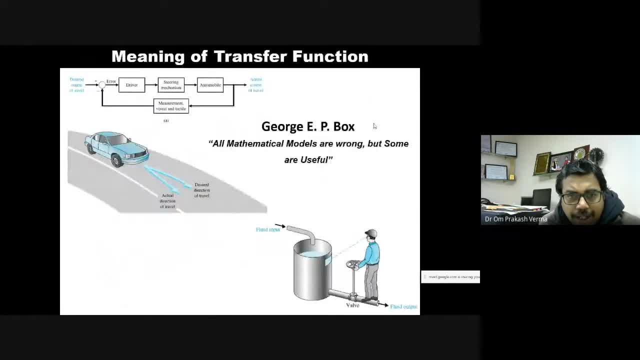 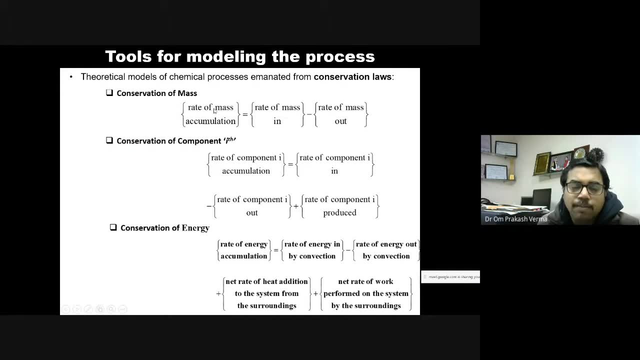 accumulation. both are the same thing, but okay, so in in minus out, equal accumulation. or you can say in is equal to the out plus accumulation. both are the same right same. in similar way you can write the conservation of component: whatever the component is going to accumulate, equal to the in minus out. 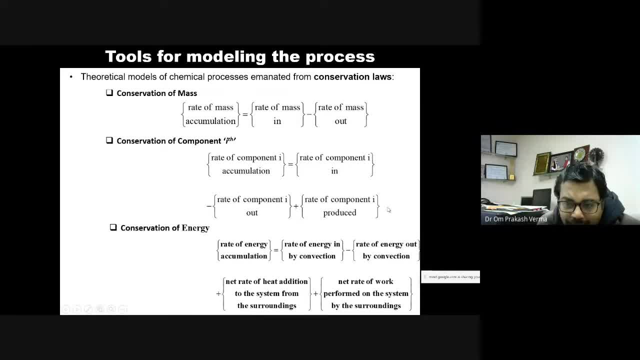 or plus component if produced, or if there is a minus term if it is consumed, it may be the maybe the minus term is also there if, the if, if, the rate of component i is going to consume. right, we have assumed that there is no consumption here. okay, therefore, only the. 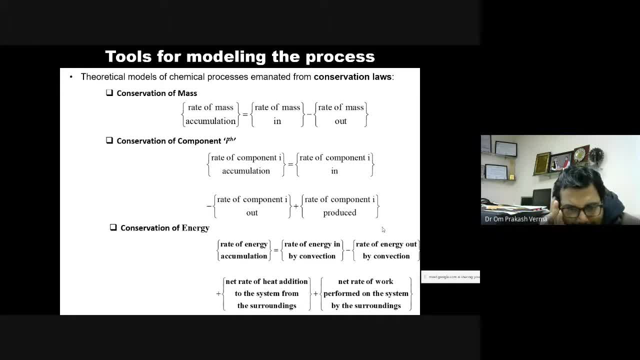 rate of component i produces here. last is the conservation of energy. in the case of conservation of energy, both the same same idea, same theoretical, same principle will are going to apply. that is equal to the whatever the energy accumulated inside the tank, inside the system, is equal to the whatever the in minus out, okay, plus whatever the heat going to the adding. 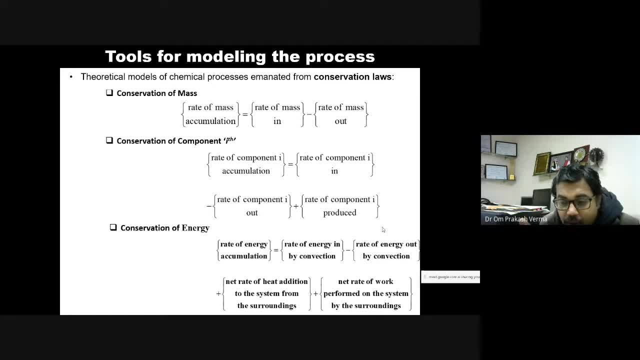 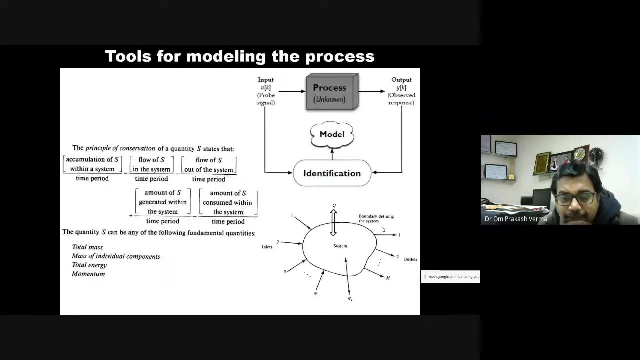 in the third system, or whatever, the heat is going to the release, to the surrounding, that all things becomes the uh: conservation of energy. right. so now the main terms is in the system, in this, here, in the figure, in this figure, that is the process, model identification, your main idea, your target, ultimate target is your control. 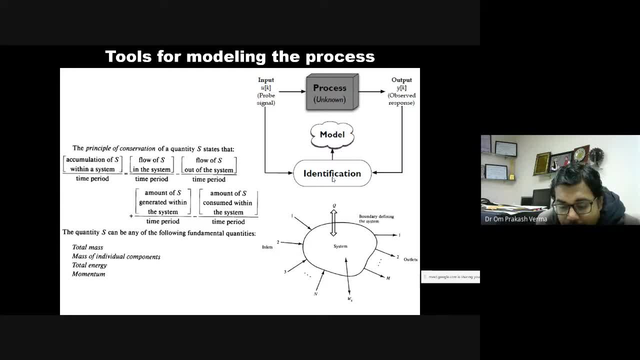 what is the control? let's say you have to going to control the level, temperature, pressure, any parameters or all the parameters simultaneously of any system. for that purpose you have to measure, you have to use control theory. okay, so in order to, in order to apply or implement the control theory, you must need some mathematical relationship between the. 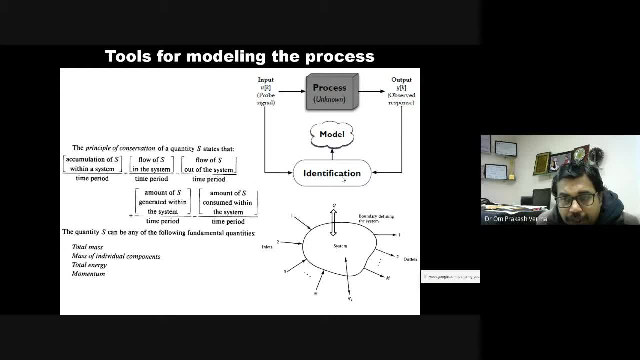 output and input. in order to that the out the relation of output and input, you must find out the dynamics and based on that dynamics we will get some transfer function. okay, we will get some transfer from the. dynamics means the process, dynamics means the dynamics of the system means it relates, the relates the output and 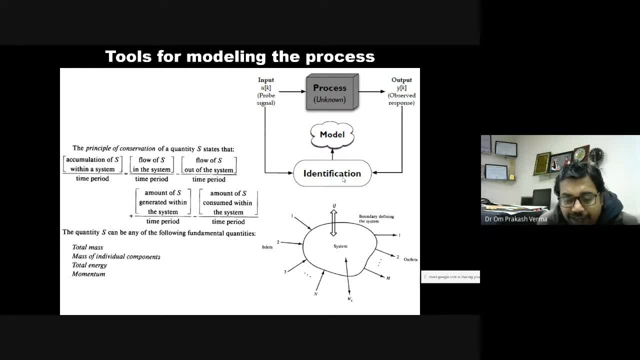 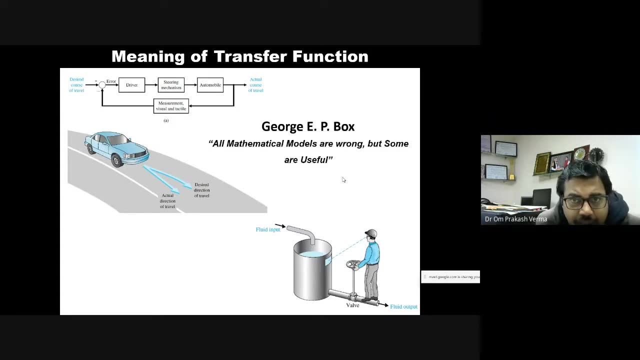 input, okay. and when we you apply some tools to the dynamics in order to simplify that, to find out the relationship between the output and input, you will get the transfer function okay. so the what the meaning? here we are going to understand what meaning of transfer function. so, transfer function: nothing. 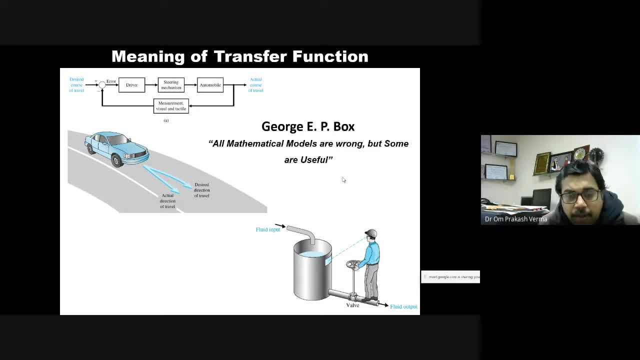 means transform. function is a relationship between the output and input. with the help of some mathematical tools, we are going to simplify the system. we are going to simplify the relationship between the output and input with the some help of some mathematical tools. okay, so you can see here. 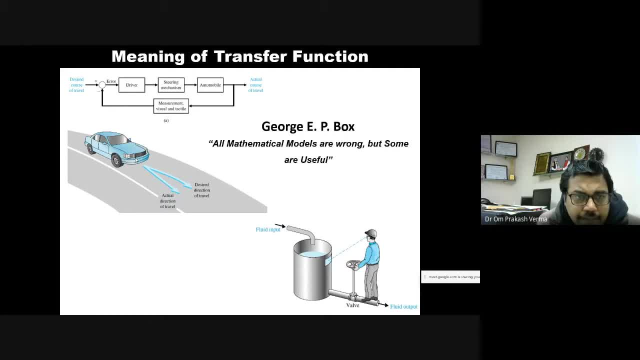 how this control theory is going to apply. Let's say this is the autonomous car or the manual car and you are going to, you know, going to some, going to going to somewhere else, okay. and let's say, suppose any how the car will drive, how you going to drive the car, okay. so let's say this is the 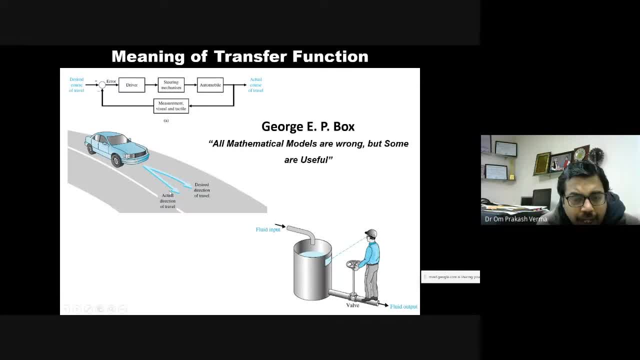 actual direction of travel is going is shown here. okay, and let's say you are going to, and the desired direction of travel is this one, okay, desired travel of this one, then you have to measure that angle and you have to, you have to change the steerer at that angle, right? okay, it is only 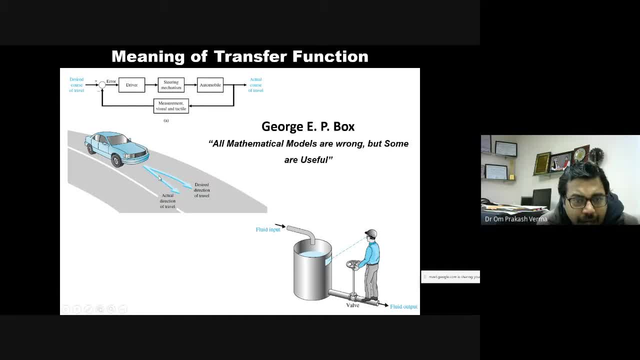 based on some measurement. so what, what? what angle you have to steer the steer, your steering right? so these are, these are the things based on this you are going to control. okay, so, and based on the same things, uh, this, this, this tank system you have to control. 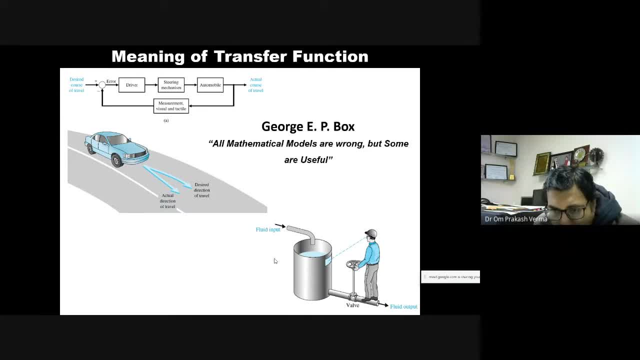 the flow of or level of this tank. so how the manual controller or how you going to control manually so you can see here whatever the fluid is going to going to inside the tank, okay, and whatever the fluid is leaving from the tank, you have to control by the help of some sensor with. 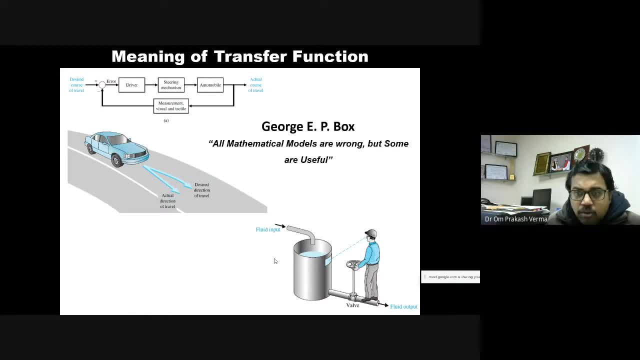 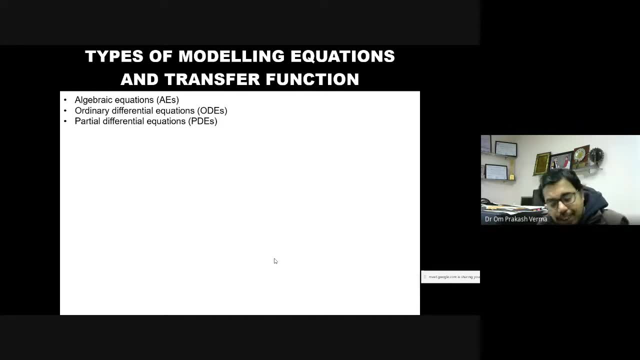 the help of major feedback system. right. so now, different types of modeling, equation and transfer function. right. so we will see, with the help of some examples, what are the natures, what are the different mathematical equations, what are the behavior of that mathematical equations we are getting. so these are the thing, these are the three. 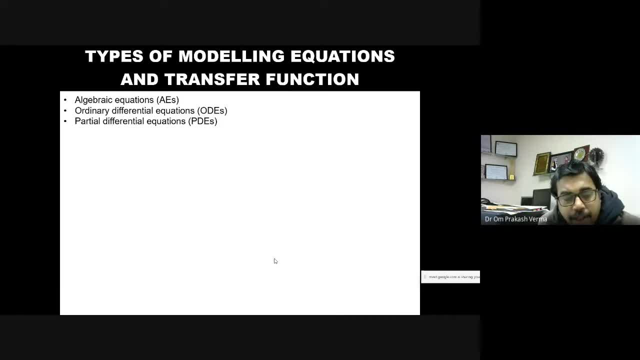 particular equation we will drive in order to find out the mathematical dynamics, or you can say the process dynamics. first nature was, first nature will be the algebraic equation. okay, so till now you have seen in the control theory, if you have developed the mathematical model of any mechanical system, 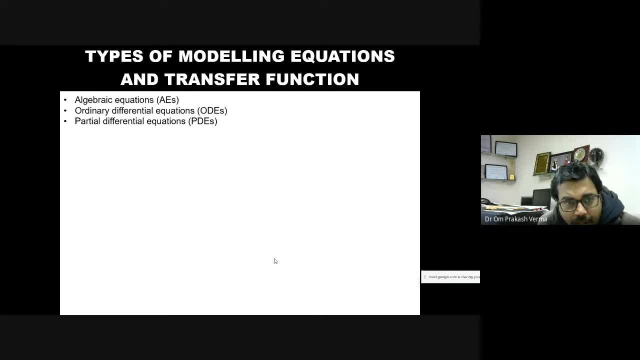 at that time, you have seen, you have encountered the algebraic equation or the differential equation, ode or the algebraic. if you are dealing with the acid state equation, then you have got the algebraic equation. if you are dealing with some- uh, you know- mechanical system, some, uh you- 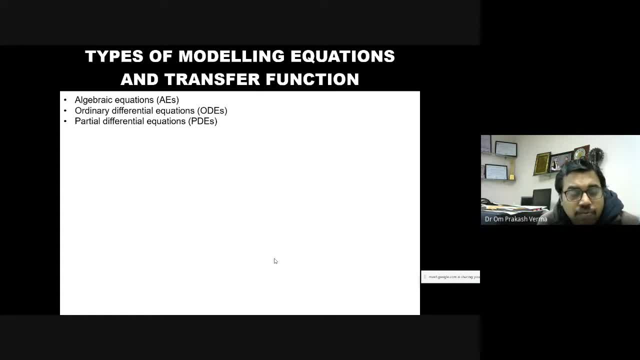 know uh dynamical system. then you will got the first order differential equation and third type is the partial differential equation. so partial differential equation is generally encountered with the distributed system. distributed system and ordinary differential equation is generally occurred with the lumped parametric system, whereas the parametric partial differential 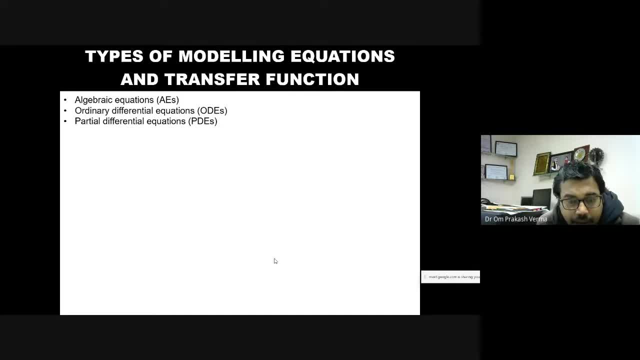 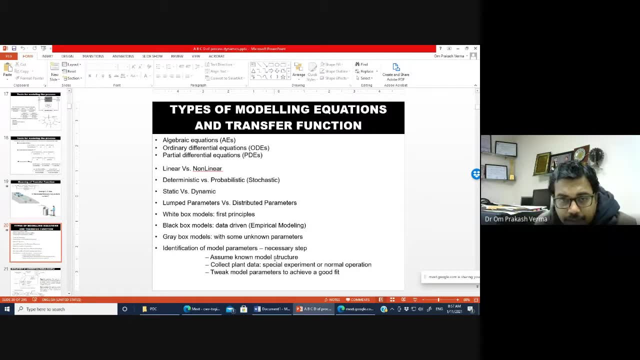 equation is comes with the distributed parameter. so now my question is with the heidi: what is the distributed parametric model, please heidi? roll number 23, roll number 23: yes, sir. what is distributed parameter model? please elaborate, I will tell you. whatever you know, whatever your idea, please tell roll number 23, heidi. 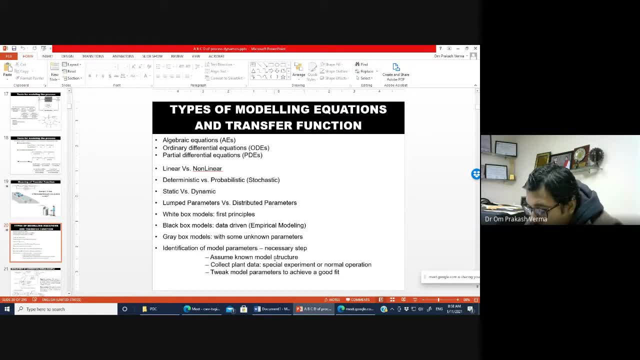 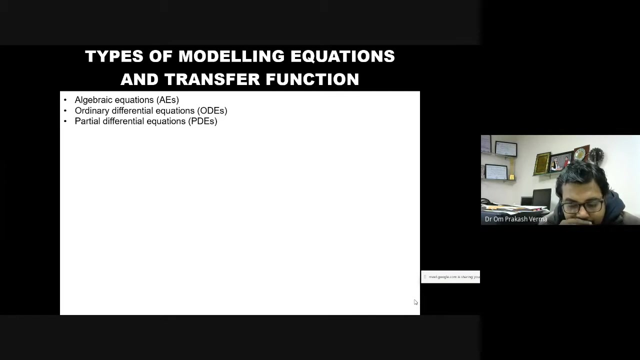 control is distributed. okay, roll number 25 in the gypsy heidi. please tell you whatever is distributed parameter. model one: quick Chang chandРЕL opening chanden. one. one 000 0000 cum one 20 jeuh 岡 h 23. 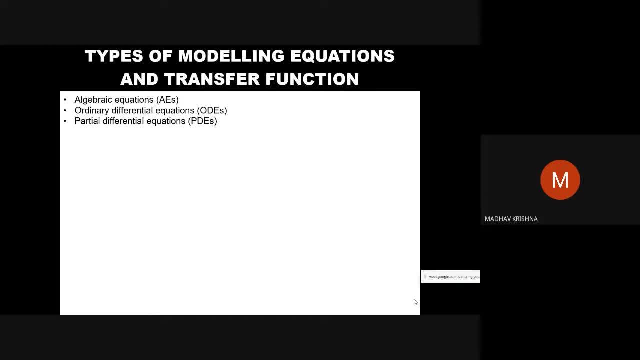 21, 2, 28, 23. How much is it changing with one and the other? so that's where the distributed parametric is, Sir. the lumped parameters depend on the time and those that are distributed depend on the time and space- both of them. 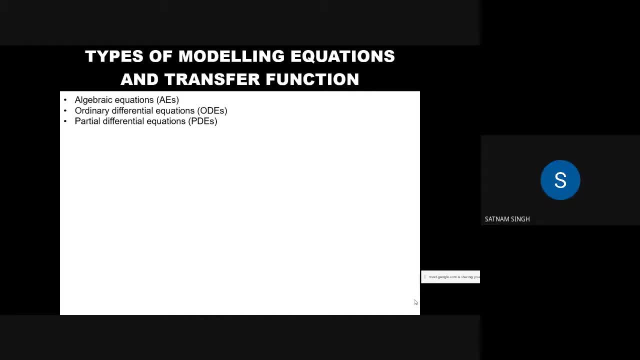 Who is this? Who is this, Sir Satnan? sir, Very good. Did you see him from somewhere or did you remember him? No, sir, he was in MFT last time. Yes, very good, Very good. Satnan, What is your roll number? 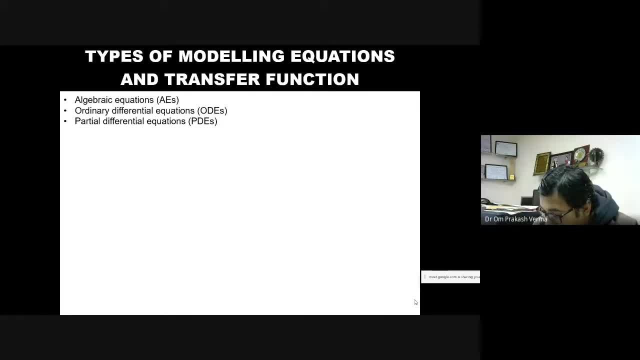 71, sir. Good, So we will see in the details of these things what are the distributed parametric model and the lumped parametric model? So point to remember is here: ordinary differential equation is going to deal with the lumped parametric model. 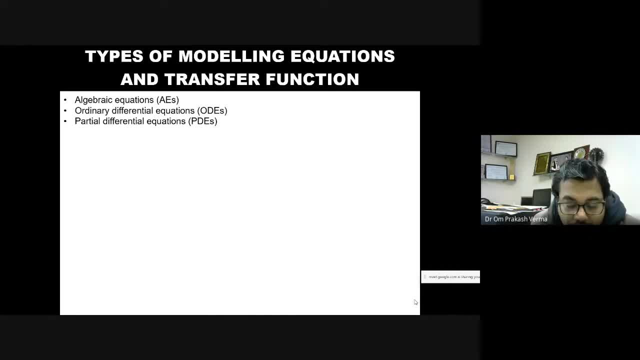 And PDE is generally encountered with the distributed parametric model. nothing else, Okay. Next type, next model. next different types of model is linear and non-linear, So we will see the nature of how the non-linear will come in the system. Okay. 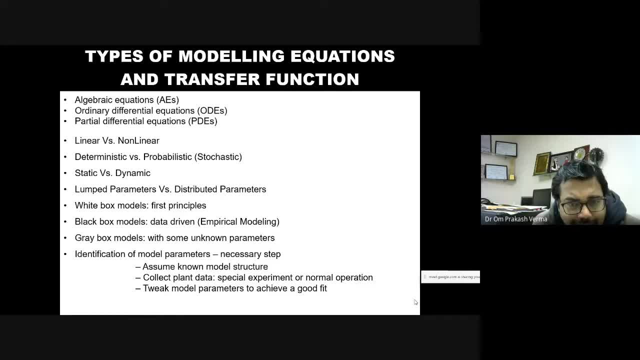 So there are two types of model: linear and non-linear. Next is the deterministic and probabilistic, or probabilistic or stochastic model. Okay, So, in order to find out the, let's say, stock market exchange. Okay, So it is very difficult to find out the model of the stock variation in the stock market. 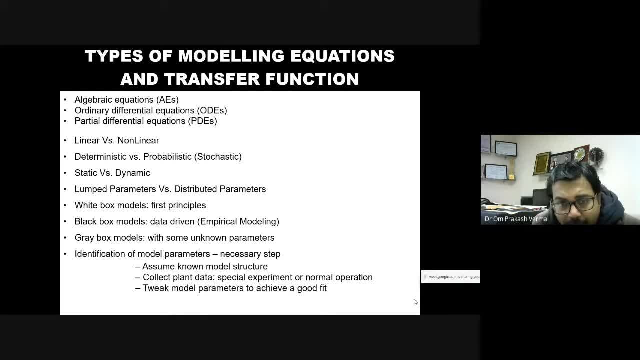 Or you can say the suppose that if a pattern of the rain in the, in the, in the per year, So if you want to model this pattern of the rain throughout the year, it is very, you know, very tough to find out the model of this eject model. 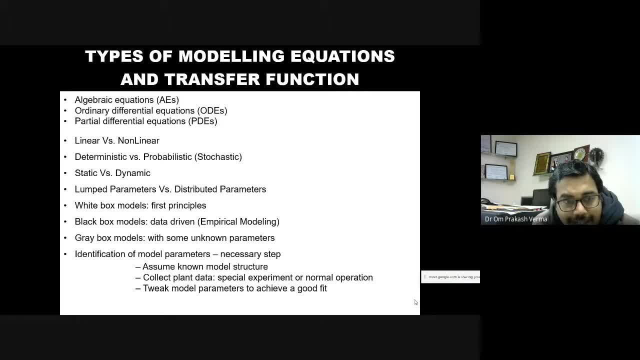 So this, this, this type of model is generally not the deterministic. This type of model is generally the probabilistic or stochastic. Okay, However, the we have seen the in the KMK process. the most of the model is the deterministic Right. 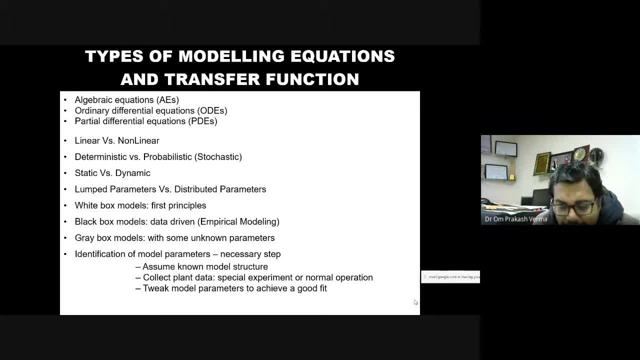 Next is the static versus dynamic. So the steady state model is the static. that is not varying with the time. However, the dynamic model is generally varying with the time. Next is the learned parameter model and distributed parameter model. This is what will make you pass. 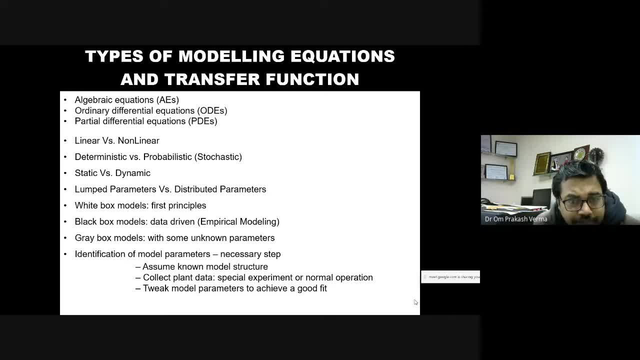 Because this is what your theory can be. There is no other theory. There is no theory in the entire PDC. Okay, So learned parameter means learned parameter means the model you are going to derive. that model is only based on, dependent on the time. 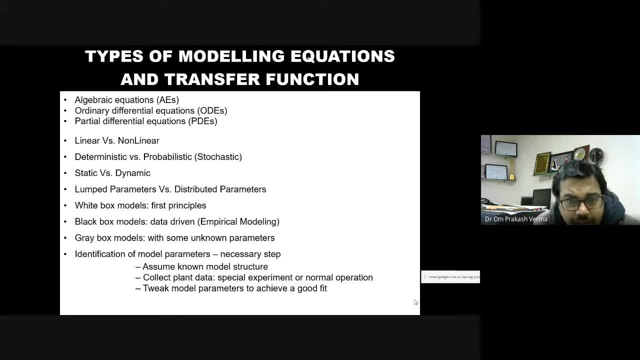 Okay, Time. Let's say this is a tank system. In the tank system, whatever the fluid is going to enter into the tank- Okay, And leaving to the tank- and whatever the accumulation. This is only dependant on the time. However, the distribution of heat, distribution of heat in in any slab. 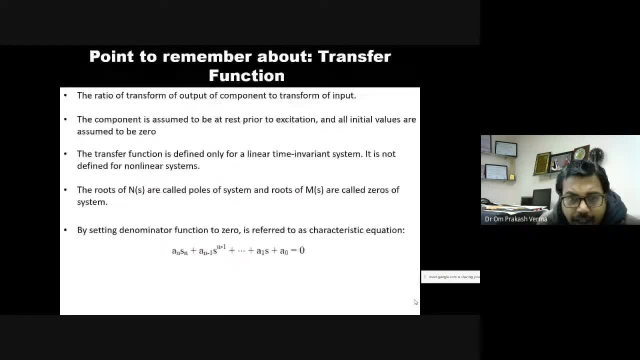 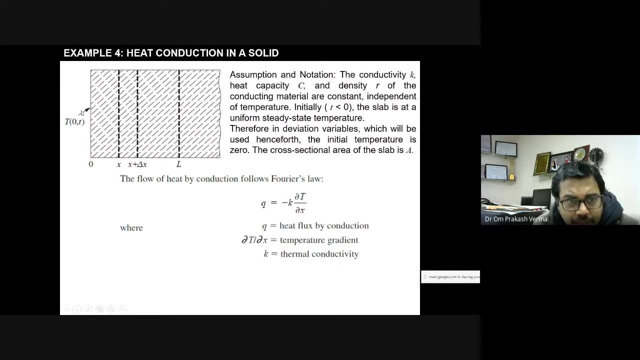 We will see later. Let's say here, In one case, I will want to show you. Let's say this one. Let's say: this is the temperature distribution. Temperature is going to distribute inside this slab. Okay, So you can see here. 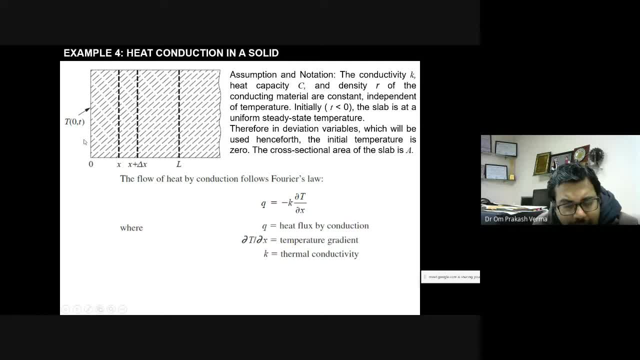 You can see here. So the time is one of the parameter Out of this, beside this time, the temperature is also dependent on this x coordinate. The temperature is at the x point and x plus delta x point. Both are the different. 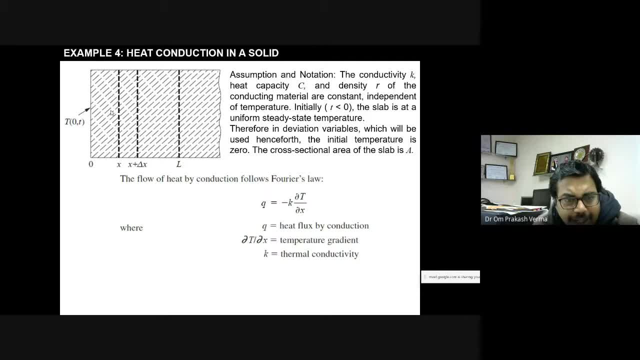 Let's say the temperature at this point: x and x plus, or y or at L. both the temperature are different, So it is dependent on the x axis or y. You can say the space. I have taken only the x axis. We can say the three dimension also. 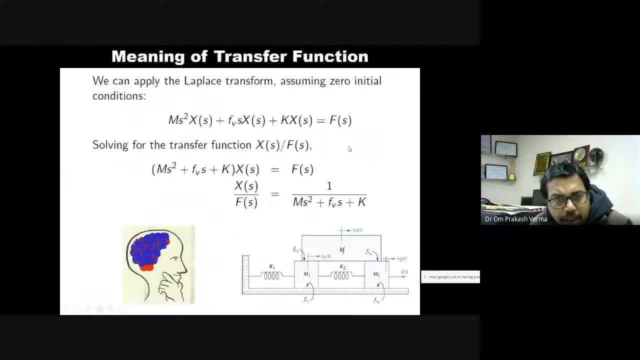 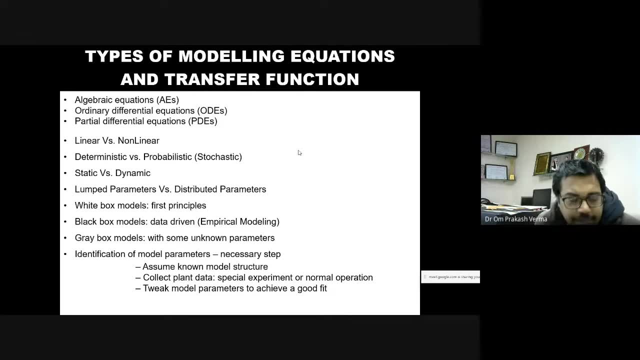 So the distributed parameter model is based on the space as well as the time. However, the long parametric model is based only on the time. Next, the white box model. White box model: generally. we derive this model using the first principle. What is the first principle? Anyone can say. 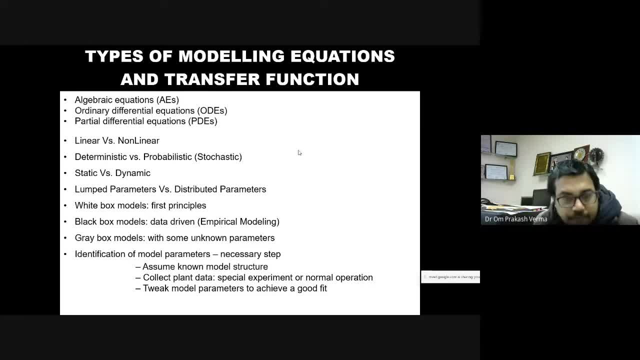 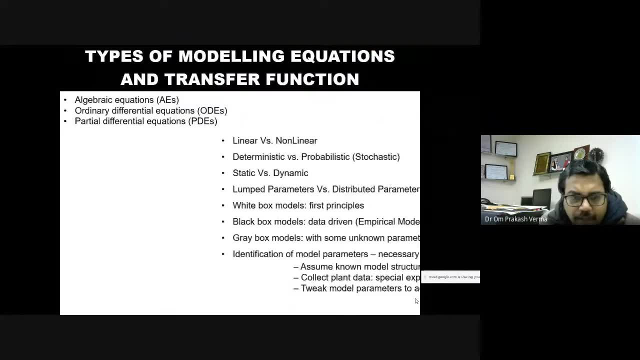 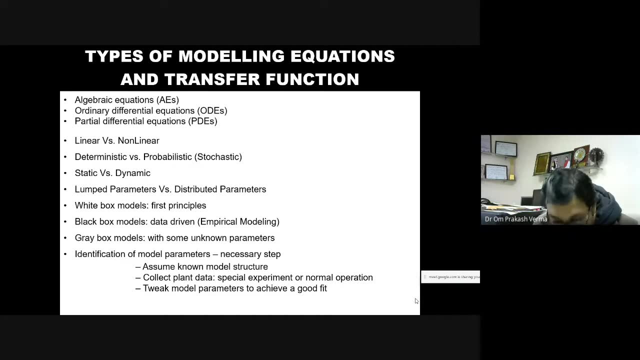 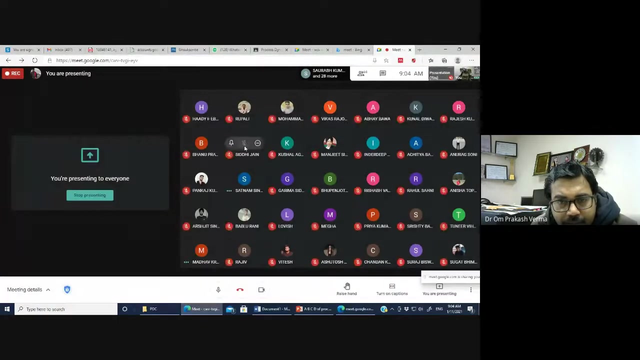 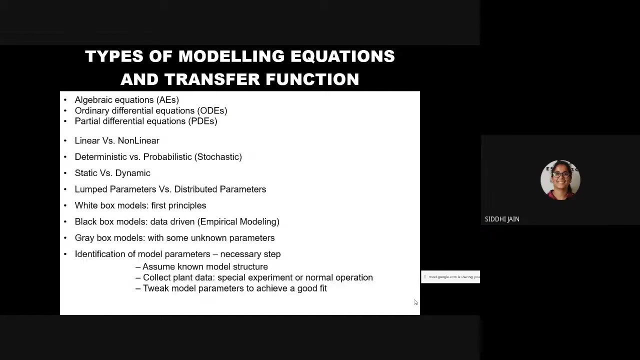 What is the first principle? What is the first principle? Anyone can say What is the first principle? Aditya, Aditya, Adity Kumar. Hello, Aditya Bolo, Shunity, Shunity Jain. 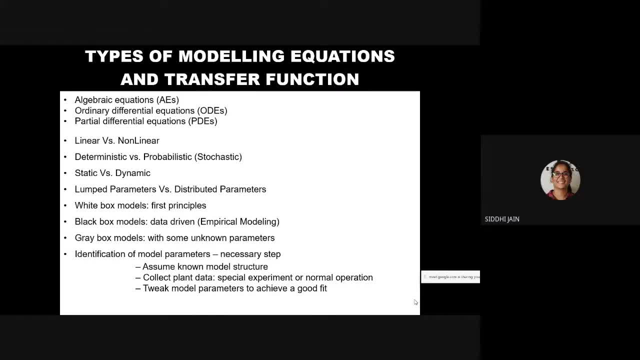 What is the first principle First? So what is the first principlevaishal? uh, any idea. white box model? no sir, have you heard about that white box model? no sir, white box model is usually the model derived with the help of the theoretical modeling, and theoretical modeling means conservation. conservation means first principle. 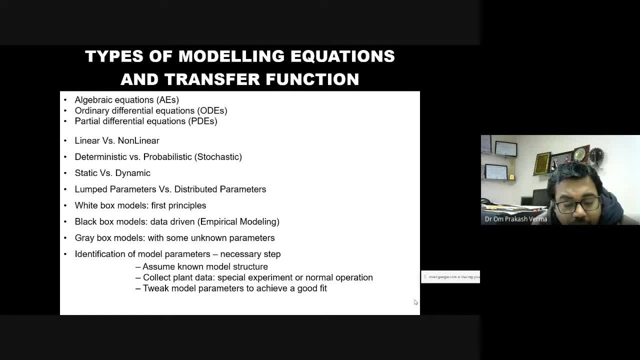 nothing else. first principles is here used for the term: principle of mass, principle of heat, principle of momentum, principle of energy. okay, conservation, so principle of conservation. conservation is no, also known as a first principle, right? so the model derived with the, with the help of that first principle, is known as the white box model. however, the black box model means we don't. 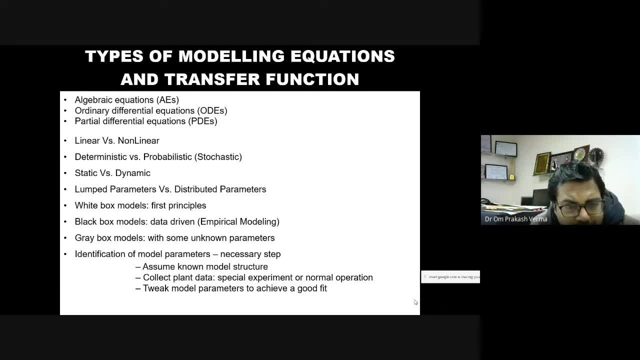 know about that model. we don't know the nature of the behavior of the input and output. so the tools using for the model of such system is the empirical modeling. so we will send some input and observe some output, okay, from that system. so based on that history of that input and output, we 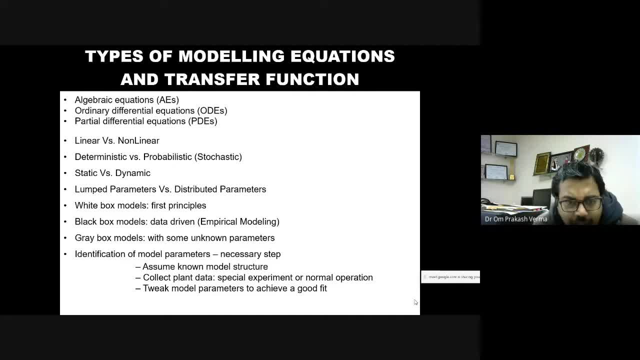 are going to develop some models. that model is known as data driven or the empirical modeling. okay, and we are going to use the statistical tool in order to develop the data driven model or the empirical modeling. the tools is the statistical or the data sense, nothing else. generally, the regression model is going to use. we will see one example. 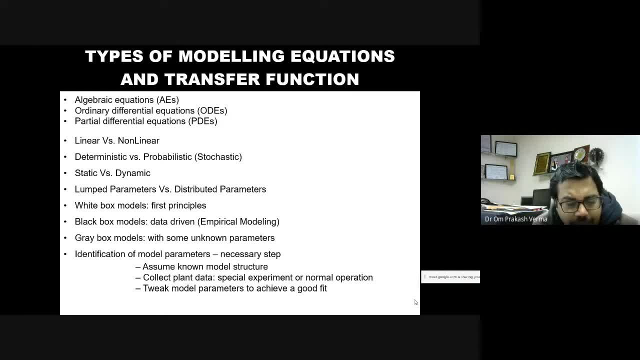 after some time. third is the gray box model. gray box model is basically: some parameters are known, some some models are. some parameters are known. so we are going to combine both the principle, the larger well being, surface, parallel concepts, as well as the empirical modeling and based on 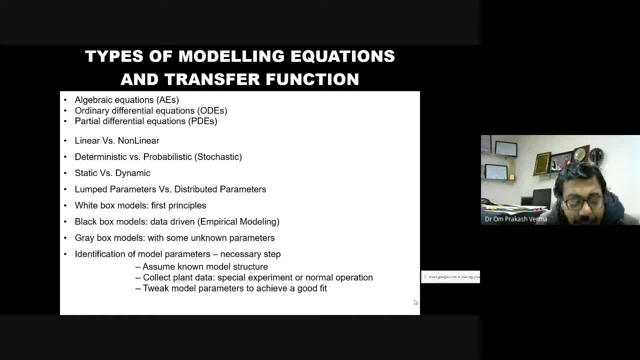 that we are, we will find out the model for the gray box. okay, so next last part of the slide is the identification of model parameters. so what are the different necessary step? what are the different necessary step when we are going to double up the models in order to find out the 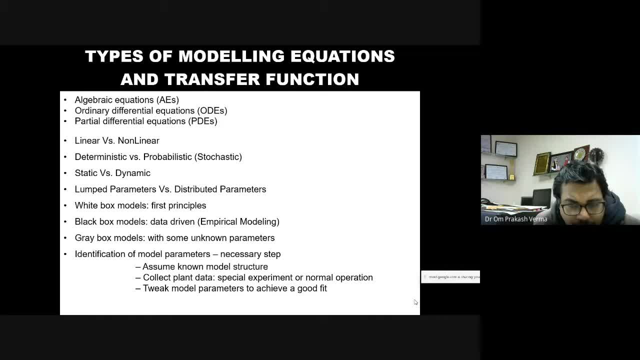 identification of the that parameters. okay, so how the identification of model parameters will do? what are? What are the different necessary steps in order to do that? So first, we have to assume the known model structure. Second is to collect planned data, or a special experiment or normal operation. 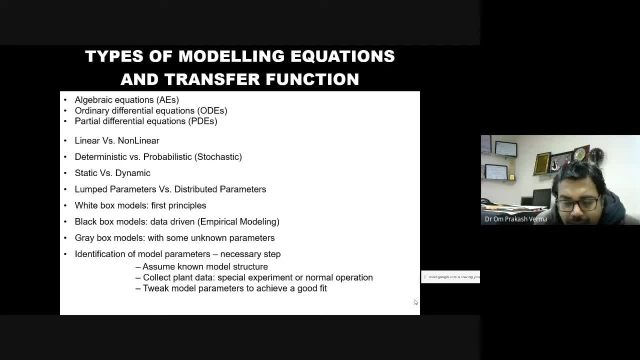 What is the meaning of the normal operation or special experiment? It means we have to assume so many things We will be surrounding. We will see after one to two minutes And the tweak model parameters to achieve a good fit. Means regression will give the line that is a good fitting. 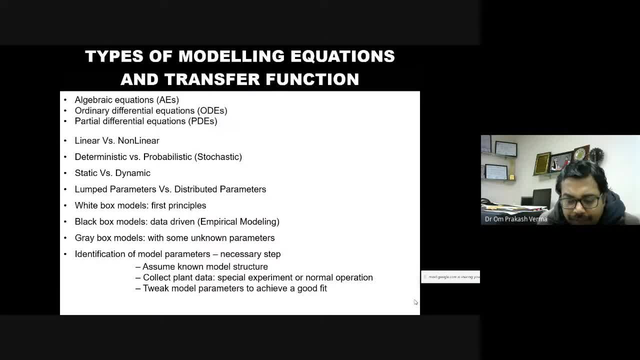 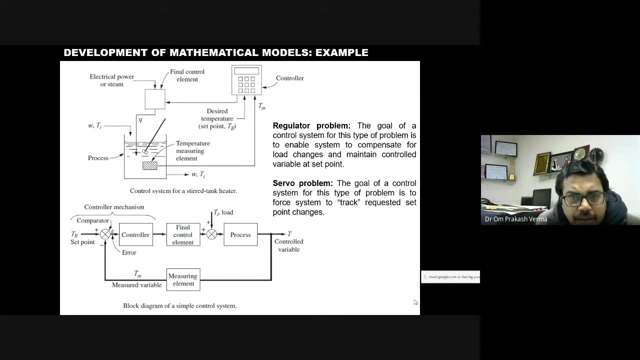 We'll see. We will test the model with the help of some testing. Testing means some tool is there on which your model is going to fit. Then only you can say: your model is fine. So first example. next is the one: 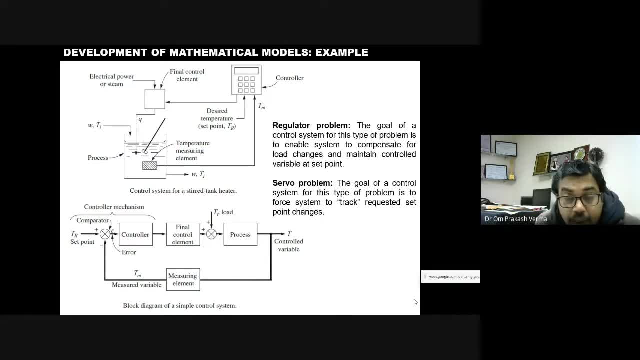 next model is also one of the model- is the control theory. This is the control theory. Let's see the control theory. First is the servo problem And second is the regulator problem. So in the regulator problem, and what is the servo problem? 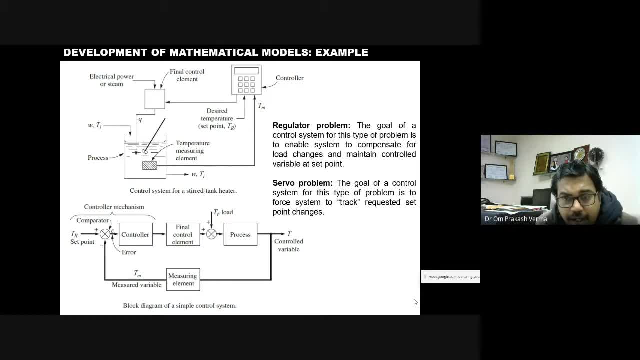 you have to understand. it is very important and generally asked in the examination as a theoretical point. So what is the difference between the regulator problem and servo problem? See here, let's say you are going- it is the feedback system. This is the feedback, one of the feedback system. 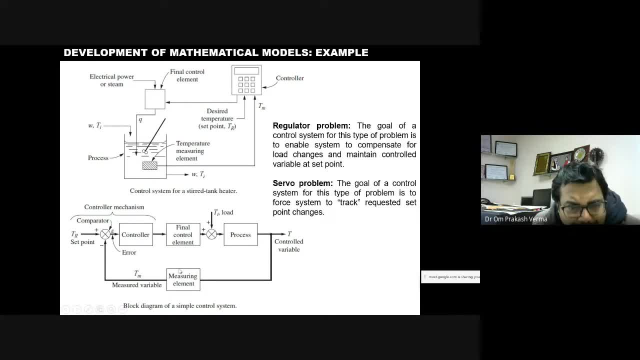 the control system. so anyone can explain this two block diagram: first block diagram and second diagram. anyone in your class? what is going to happen here? anyone? because i have demonstrated this figure two to three times or four times anyone. in the first diagram, electrical power and steam means that it is working to give the temperature in the process. 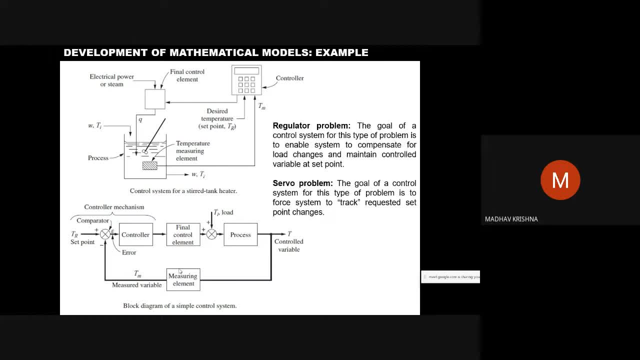 then there is the work of temperature measuring element that it will sense the temperature and read it. ultimate target is that: how much the desired temperature is, how much error is happening? whether it is going up or down, it has to be controlled by the final control element. 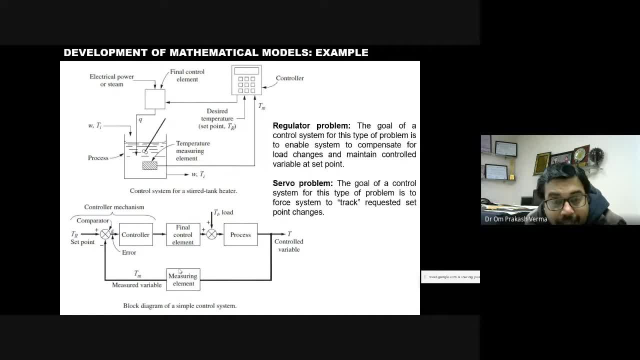 that's right. ultimate target is to control the temperature of the fluid inside the tank. in order to that, we have to measure. we are going to measure that temperature of that fluid inside the tank. that is going to leave that as a product at the ti point. okay and just. we measure these things using the sensor we send to the some controller. at the controller point there is a some summer is there. 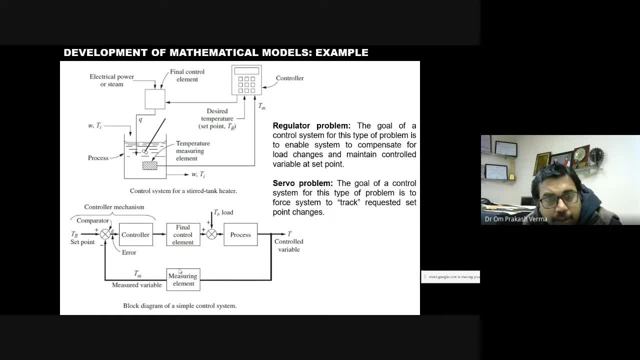 and at summer, the setpoint desired value of the temperature is going to the, going to inter that point, okay, and we going to subtract the measuring temperature and the set point or, based on that error, the final. the controller will decide how much, how much element or how much final control element, how much valve is going to open or close. 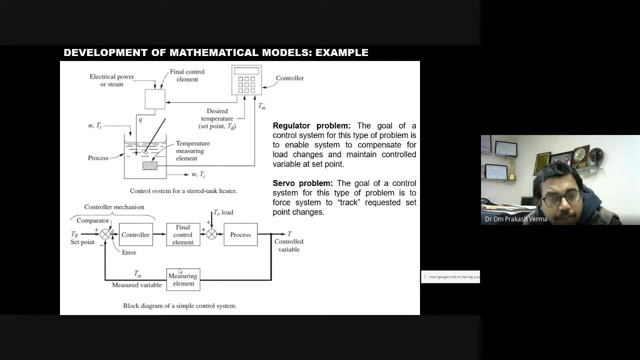 Okay, based on that opening or closing of the valve, the electrical steam or the electrical The valve, The valve is going to open or close and based on that, Okay, What is going to happen is that power- the steam or the electrical power- is going to enter inside the tank and 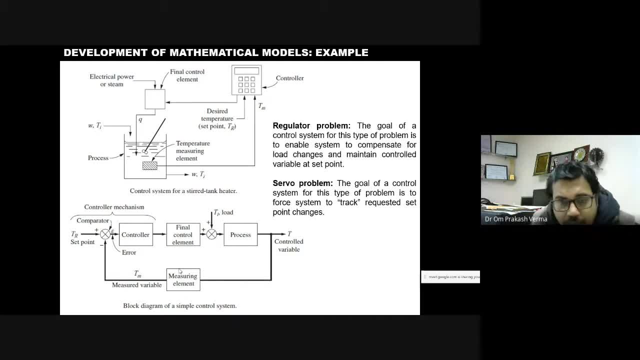 and therefore this temperature is going to control. okay, so this is the theory of going to control the temperature of the steer tank heater and same is represented in the model, in the broad diagram, right? so this has been represented with the help of low diagram. okay, now what I mean by it and you can. 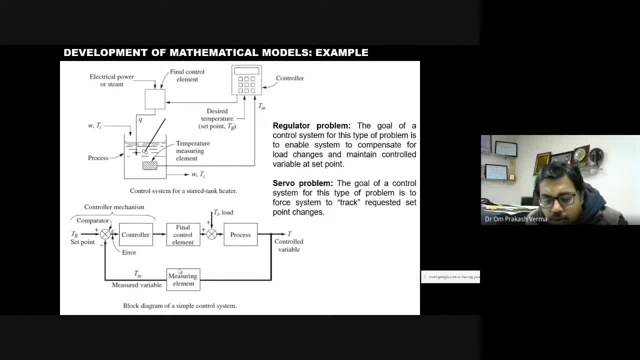 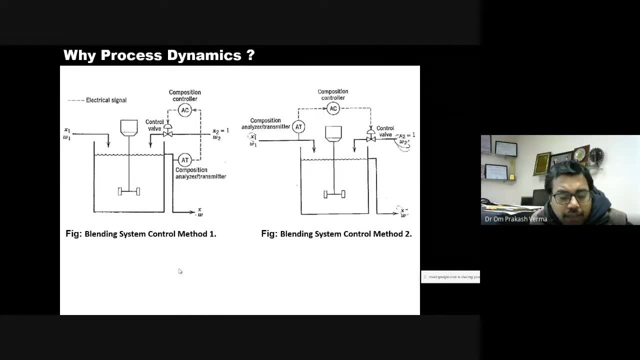 see there are the Ti. Ti is a load we have seen through. we have already understood this thing. Ti, with the help of the feed forward control. you can see here the Ti we have already understood. so if we are going to control with these, this parameters, that it will. if we have so the Ti load, okay, it is a load, this it. 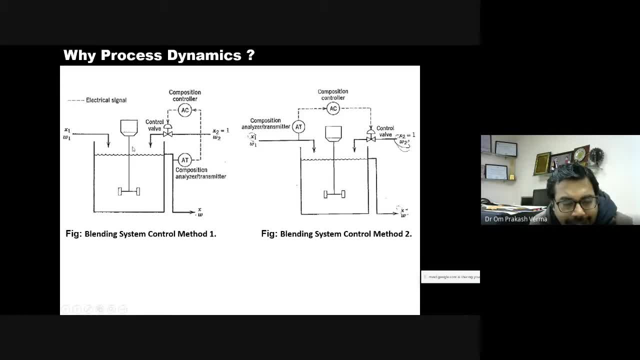 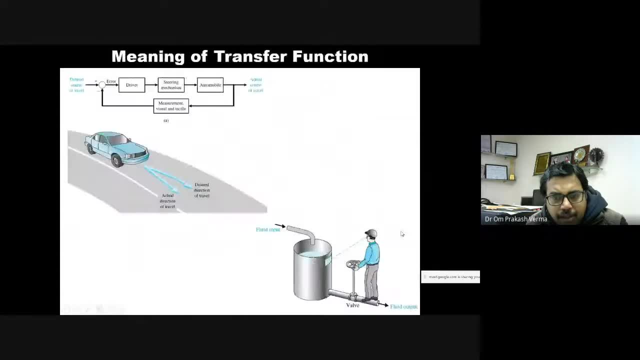 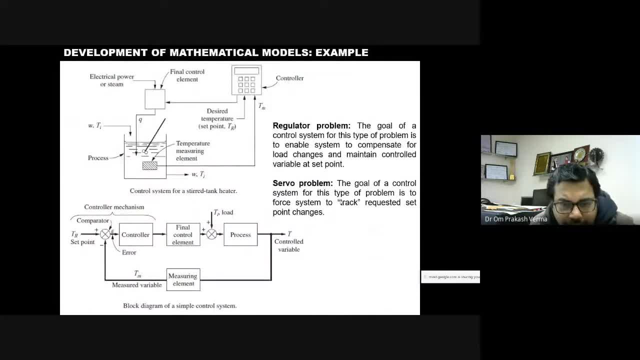 with the help of the block diagram. this is the Ti, this is the load. okay, so when this Ti what the realtor means, realtor problem means the goal of control system for this type of problem is to enable system to compensate for the load change and maintain controls variables at set point. 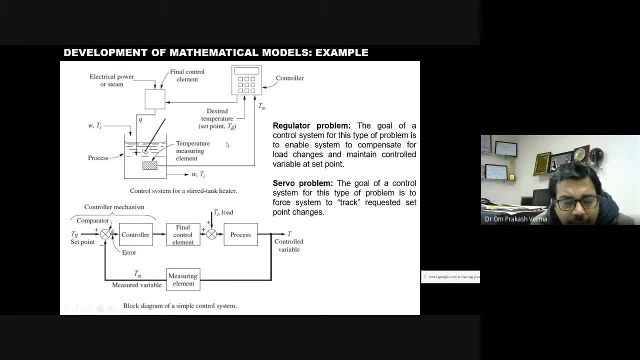 means it means for the regulator problem. you have to understand it. set point is going to the constant, the. the varying, the variation is only happening in the TI node. this will be, the will be the constant. okay, set part will not change. however, the load will change in the case of the winter problem and the vice. 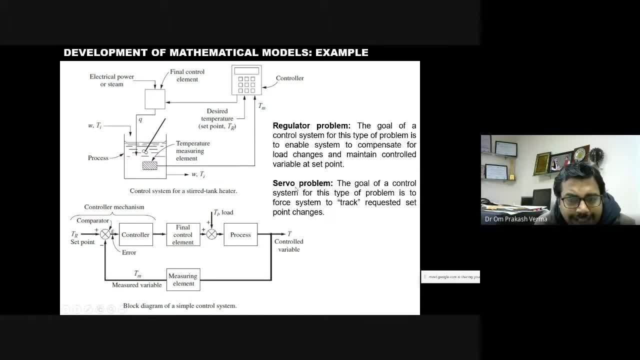 versa in the happened, the sorrow problem. the sorrow problem: it is used for the tracking purpose. tracking purpose means the state point will change. however, the load will become constant. load will not change in the sorrow problem. okay, so generally the robotics problem. the robotics problem is encountered with a 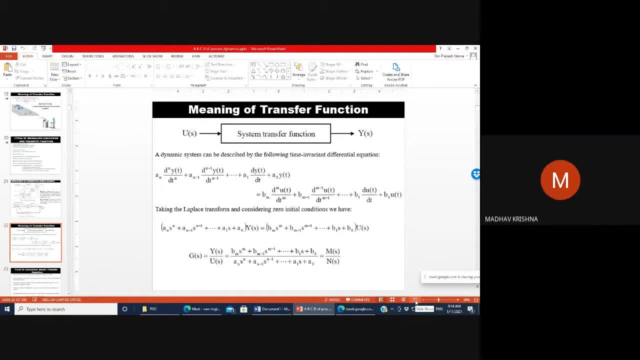 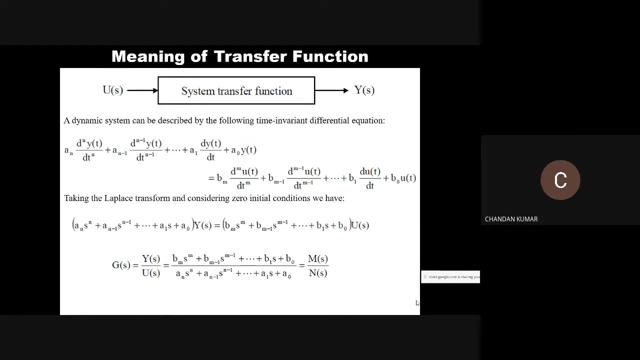 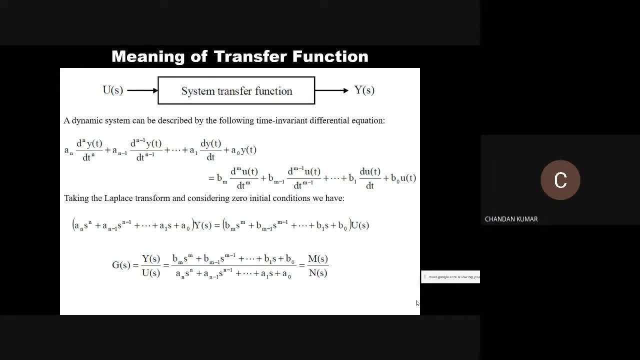 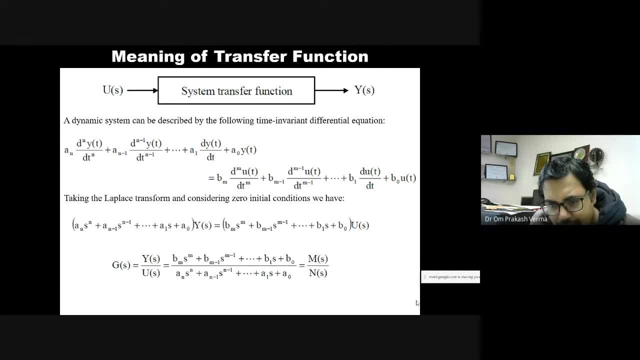 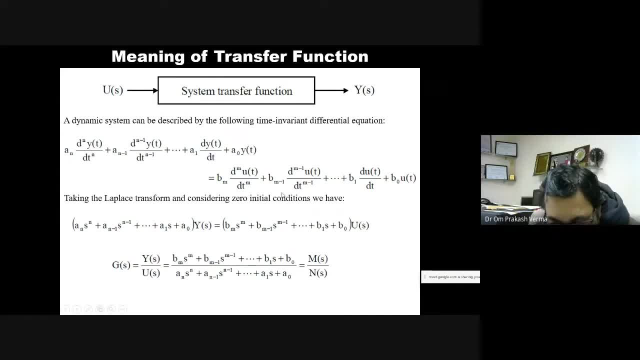 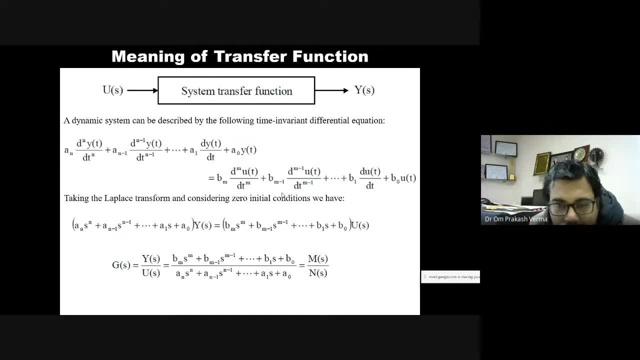 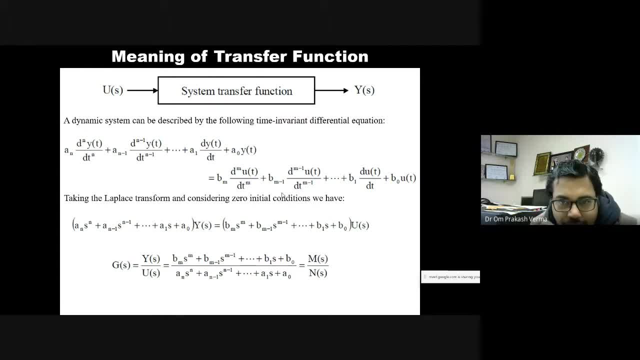 the output and input. you are going to write some equation: with the help of mass transfer, with the help of heat transfer, with the help of momentum transfer, whatever, in order to that, you are going to write some equation and that equation is maybe the first order difference of the second order of this. 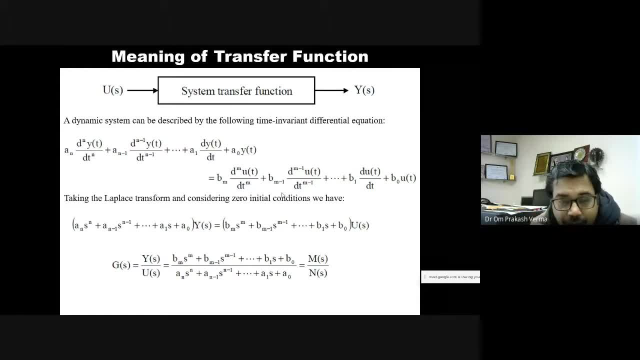 measure may be the simply algebraic equation. let's say: this is the differential equation, ODE generally, because accumulation is there. therefore, generally you are encountered with the ODE. okay, so this is the differential equation. let's say: this is the output side by T and this is the input side. you. 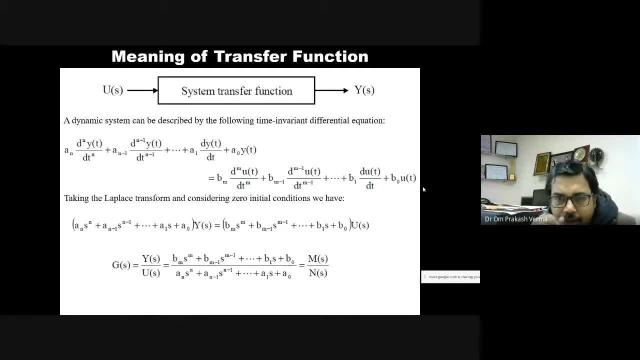 have written some equation and we have developed this type of dynamics. now, how can we relate the output and input? okay, how this output is change with the help of mass transfer, with the help of mass transfer, with the help of mass transfer, this, this input. in order to that, you are going to simplify this equation and 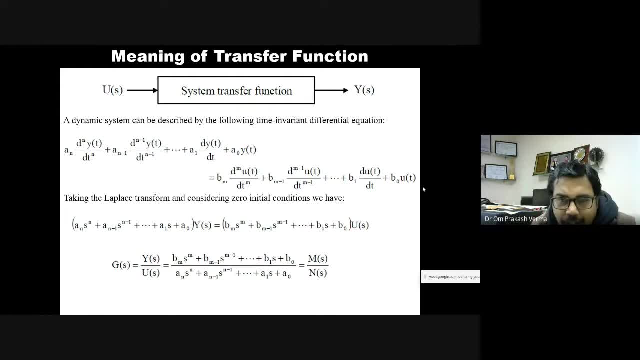 therefore, we are going to implement either you: either you find out the solution of this differential equation and you know as your differential equation becomes higher order, or there it is a tip: it is very difficult to solve the differential equation as compared to solve by solving the that differential 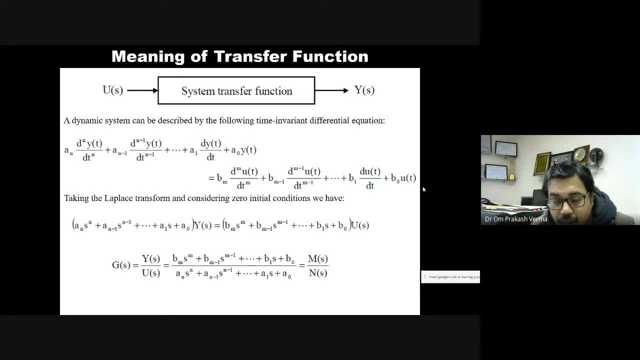 equation with the help of laplace transform or with the help of other two other tools, that is, the floor transfer. am I right? am I right or not? difference difference the difference of Vanignite in nature, or we are going to use, we are going to apply that tool. 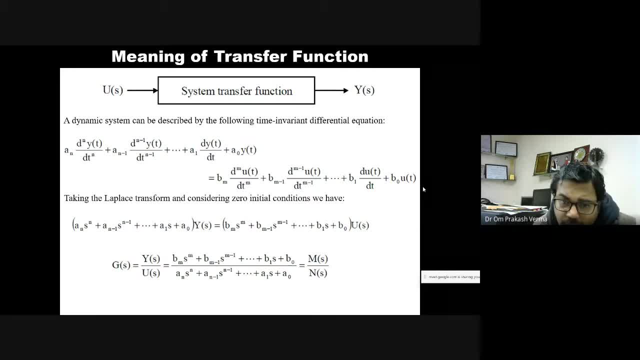 particular tool for or in order to solve that differential equation. Am I right, your? so now you have a situation- whatever equation you want, I want- in which the right answer Camill isn't, it is inBox, in Josh, Towards here, which which equation is outward to is second, and in some question- or isn't it true, because this is also Morba- 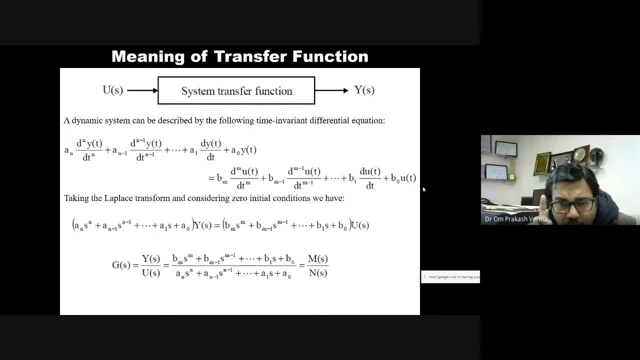 know it's order to avoid that complexity in the differential equation, we are going to use some tools. ultimately, we have to solve this differential equation and find out the variation of the Y with the help of input and the time. nothing else, okay. in order to in order to that, just, we're applying some tools for solving or. 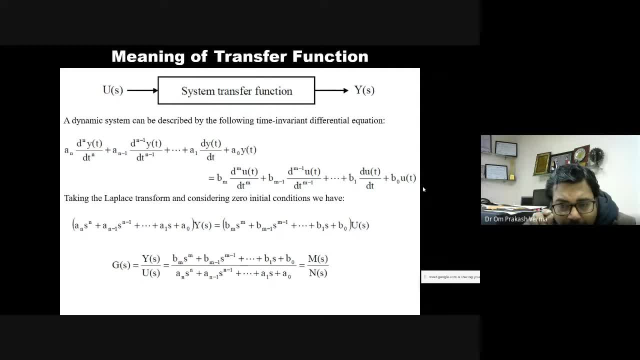 for you know, you make your, is your, make your, you know complexity easy, nothing else. and therefore we're going to apply some tools and therefore that Laplace transform or the Fourier transform or the J transform will help in that, nothing else. now the question is, why not? we are going to use the Laplace transform or the J? 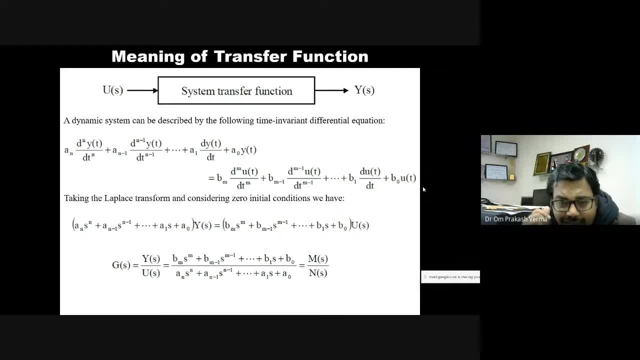 transform, J transform is used for the discrete system and this is the. this is the continuous system. differential equation is written for the continuous system: yes or no? yes or no, and when the system is the discrete digital, at that time the, let's say, R max model, auto-relation model, auto-relation moving. 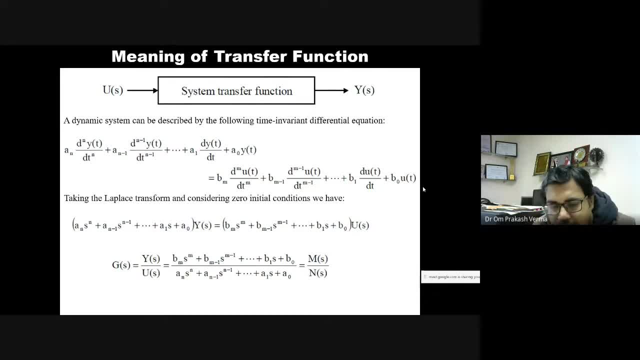 average model model. all these models are the discrete model and that place will encounter with the J transform, nothing else. at that place you are defying the top, the lap, the T测 function with the help of J transform, nothing else. so for use of your last transform and full, you're responsible. most are most. two are the: 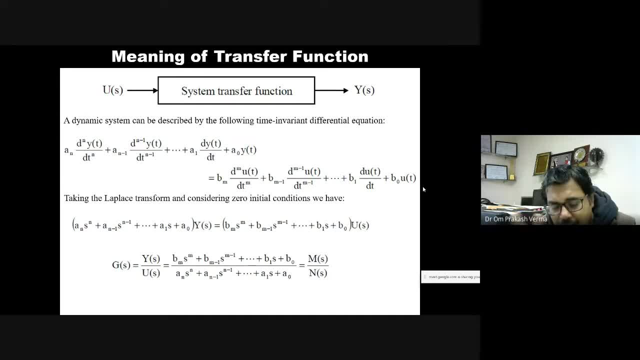 very, you know, you can say, you can say it is very near level of example arrived, similar level, nature of laplace transform. but these are not. these are the entirely different tools due to some, uh, you know, uh, the converging nature. okay, converging nature, which different. 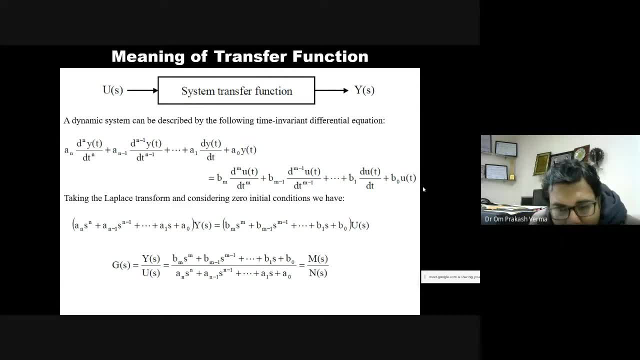 nature. unfortunately we have not studied in the previous semester fourier transform. okay. so question is why we are going to use the zero initial condition. it is only one question now. if you are not making the zero initial condition, the system becomes non-linear. why we will see with one example. okay, that's, let's say, of dy by dt, dy by dt plus y, equal to five. 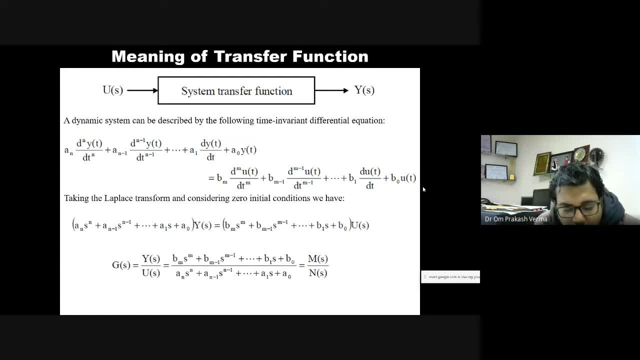 other equation, let's say two into dy by dt plus y is equal to zero. so this is a non-linear equal to five equation and you have to find out the, let's say, differential equation: five x x t, five x t, this side, the y t and this side in the right hand, in the right hand side. 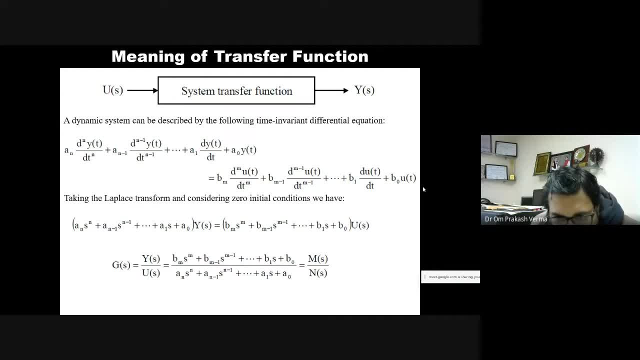 the x t and the left hand side the y t. five dy by dt plus y t equal to x t. let's say this is the equation. so when we are going to apply the laplace transform then divided by the laplace of dy by dt s into y t. 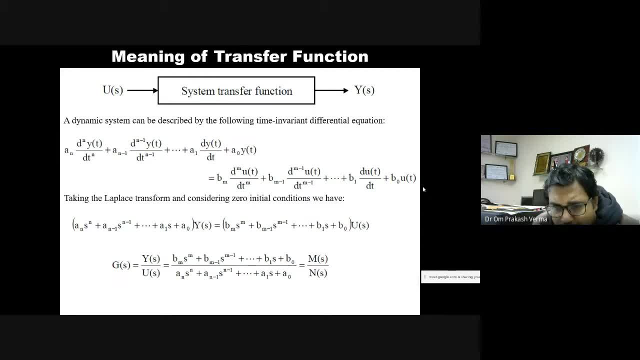 ys minus y, zero, minus, am i right? what is the laplace transform of divided t? yes, sir, repeat s into ys minus y, naught y, naught y to y, naught initial condition. that is the initial condition, okay, let's say the initial condition, okay. so this is the s, ys, okay, and the laplace transform of yt is y, s and the laplace transform x, t is. 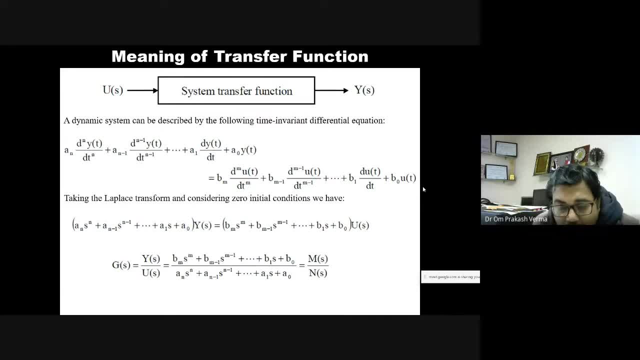 xs. but due to this y0 minus, you are not able to find out the output and out input relation ys upon xs. you will never be found. found, yes or no? yes, sir, minus, okay. the y0 minus will make the system non-linear, okay, and therefore you're not able to find out the laplace transform. 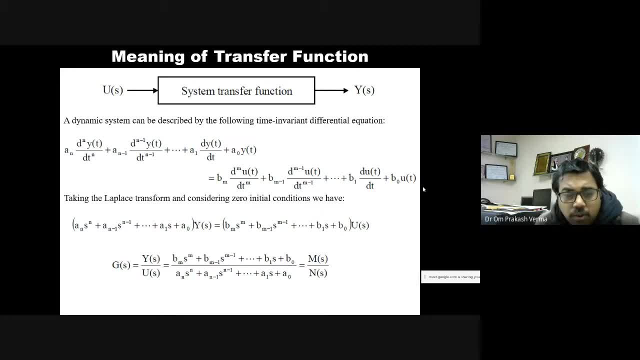 output and input. okay, so, therefore, we are making, we are assuming that the, we are considering that initial conditions would be zero. okay, exactly, exactly because, because, because we are using the state of space equation, okay, and this is the, this is the, this is the, you know, the restriction, judicial condition. 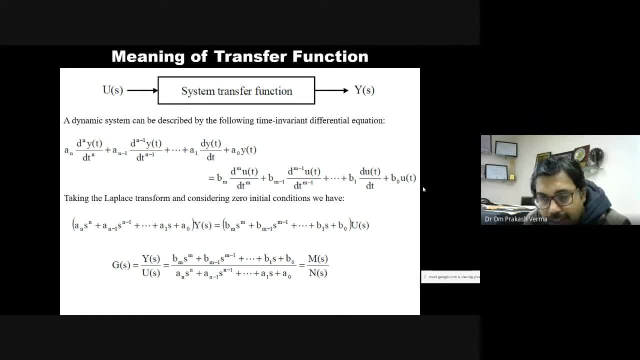 okay, there's a disadvantage of the system. we are. no, we don't know the exact nature, but, however is very harsh. you are going to study the tools in the control theory for the for the different tools for the study. okay, so in order to learn that tools, we will study. 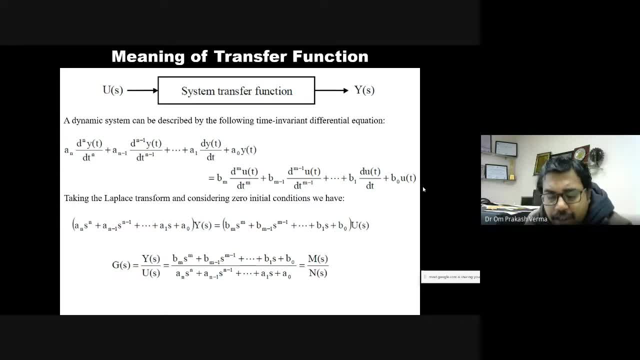 to the linear theory, linear time, invariant theory, because your aim was not to understand the process. your aim was to understand how the tools of control theory are implemented. let's say, if I started non-linear theory directly and applied it directly to non-linear theory, like this, you would not be able to understand. 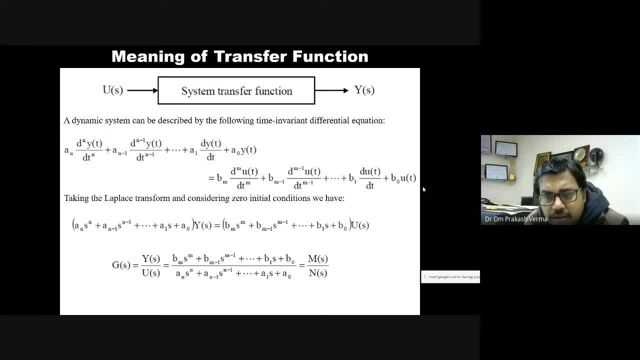 therefore, for ease to better understanding, we have encountered with the linear time invariant system. however, it is also true. the linear time invariant system in practical never exists, but the theory will remain same. ok, the theory concept will remain same. so to understand the concept, you have to understand this. 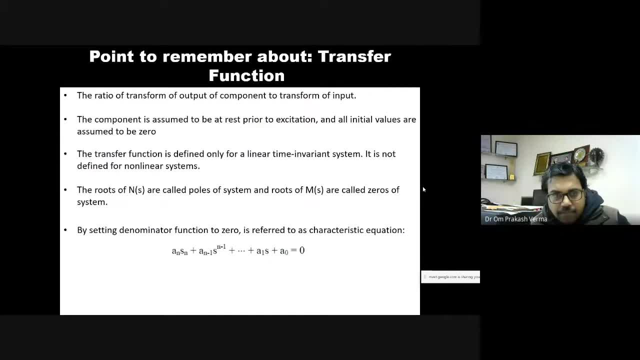 ok, is it clear? ok, so you are trying to remember. this is the last slide of today. ok, trying to remember about the transfer function. so what is the transfer function? this is the generalized equation you have, you have already this. you have you know, reading. read it on the. 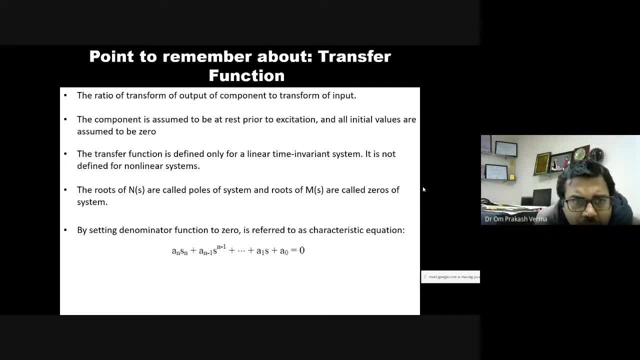 the books to the books line. ok, so what is the transfer function? transfer function is nothing else: the ratio of transform of output, of component to transform of input. ok, so the component is assumed to rest prior to excitation, that all initial values are assumed to be zero. 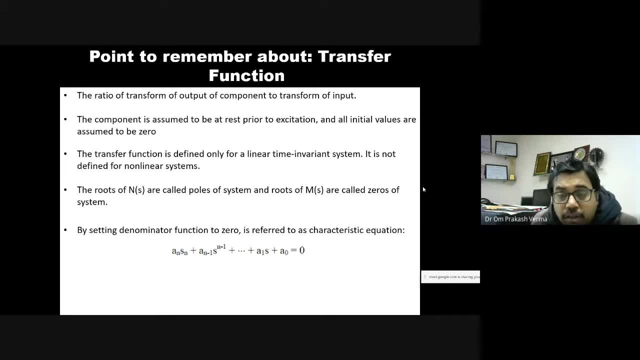 so the transfer function is defined only for the LTI system. why, I have told you, it is not defined for the non-linear system. for the non-linear system, we will handle with the different tools. ok so, but we will see. we will make the non-linear system. 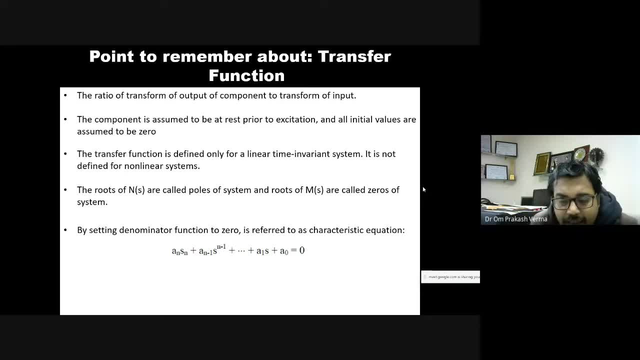 into the linear system. there is also tool, because studying the linear system is much easier. ok, so for the non-linear system, we will study how the non-linear system, we will study how the non-linear system will handle if the non-linearity is not much higher. ok, 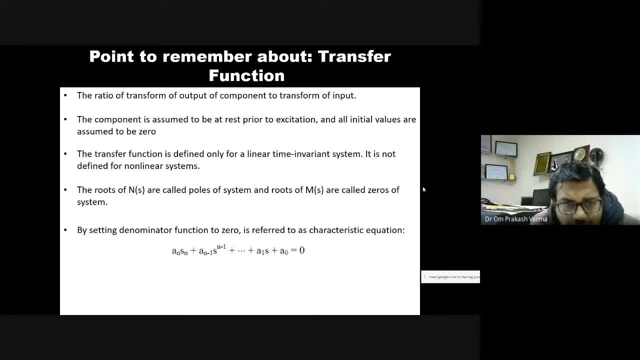 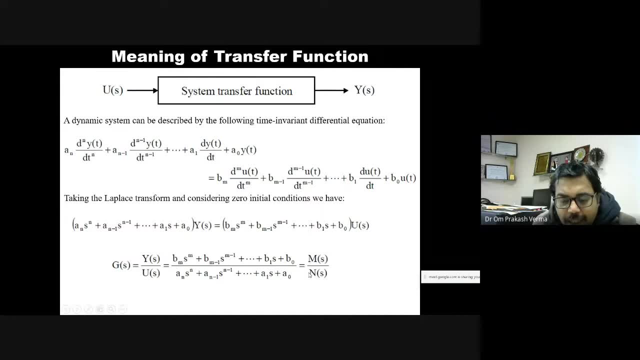 we will see the root of n. ns are called poles. it means ms. if we find the root of this, we will find the root of ns. whatever the root of ns is there in the denominator, this will be called the poles. however, the roots of the ms, this polynomial, 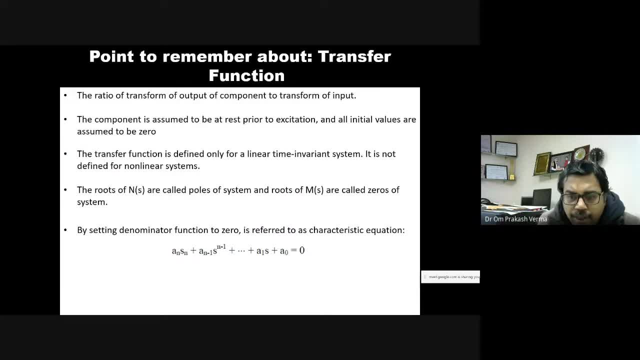 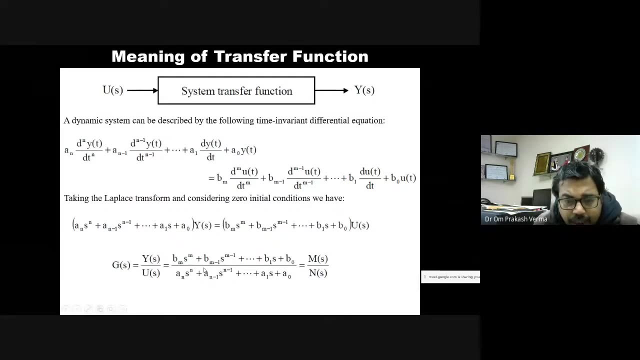 is known as the zeros of the system. right, so we will see how the non-linear system will handle the non-linear system. ok, so what is the characteristic equation? the characteristic equation means, by setting denominator function to zero, means means, if we are setting this equal to zero,